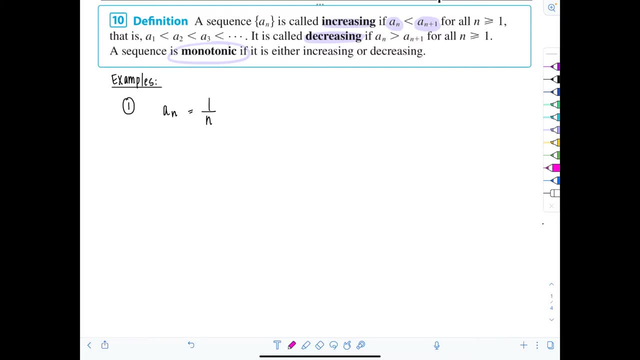 by using the inequality here and comparing an with an plus one. So an we know that that's just one over n. An plus one would be one over n plus one, And it's pretty clear an plus one is always going to be monotonic. So if we're going to compare an with an plus one, we're going to 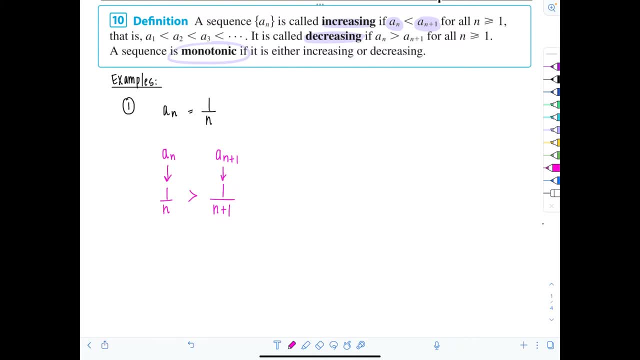 be less than an. So look at the definition here which one applies. If an plus one is less than an, that means the sequence is decreasing. So you can just say this implies an is decreasing And this inequality should be pretty straightforward for you guys to establish. 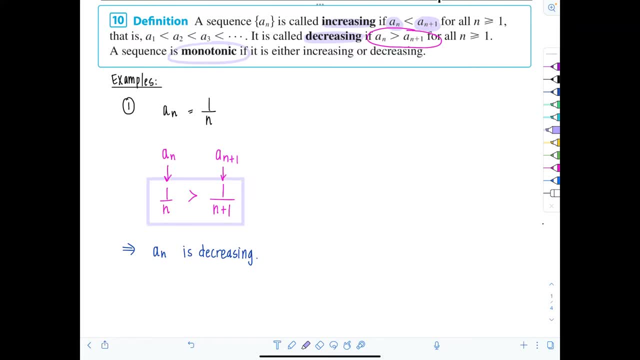 Because, notice, both terms, an and an plus one, are monotonic. So if you're going to compare an with an plus one, just have a one in the numerator. The only thing that's changing is the denominator, And it should make sense if the denominator is larger, like it is here: n plus one. 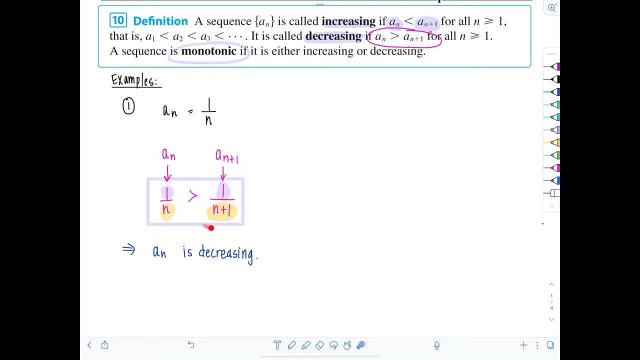 that's bigger than n, then that means this overall expression is smaller, right? If you're dividing by a bigger quantity, So you can just go ahead and directly use the definition that way If it's a little hard to see which way the inequality should face and you're not quite. 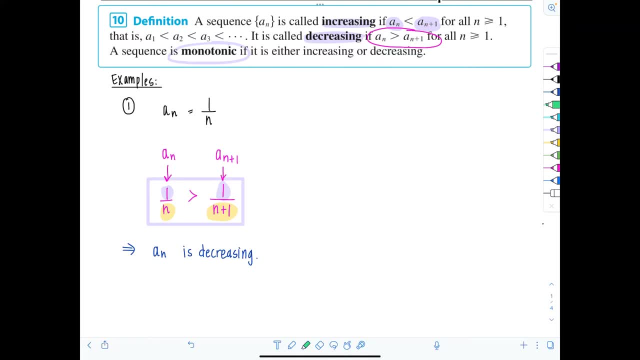 comfortable with it, then you can just go ahead and divide it by a bigger quantity, And that's it. You do have another option. So think back when you were in calculus one. how did you show a function was increasing or decreasing? You would look at its derivative. Now, just be careful with 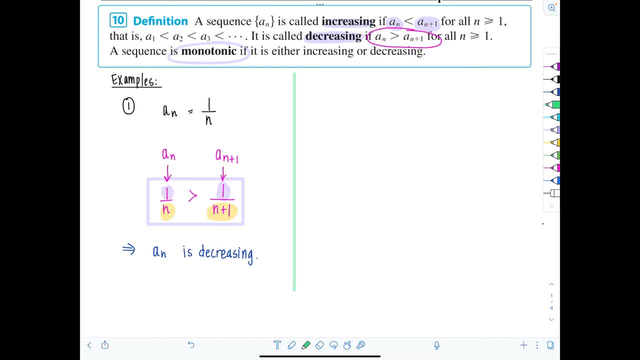 your notation, though, Sequences are not differentiable. So if you're going to bust out a derivative, make sure you define a function first. So you're just going to say: consider a function f of x equal to f of x. So if you're going to bust out a derivative, make sure you define a function. 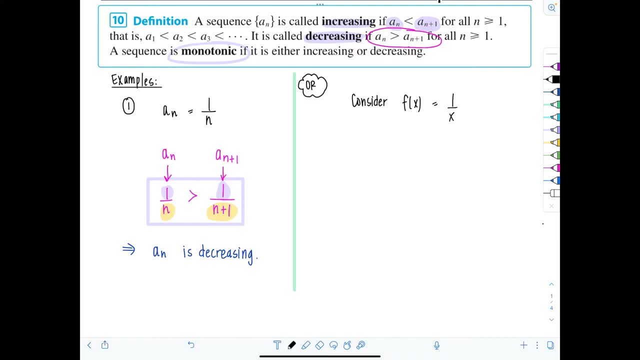 to one over x. all right, So just replace n in your sequence with x and define a function. And I know I'm going to take a derivative. So instead of one over x, I'm going to think of this as x to the negative first. okay, So let's go ahead and take the derivative f, prime of x. 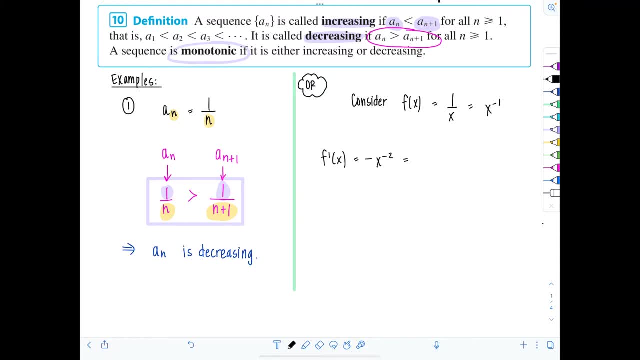 That's going to be negative. x to the negative. second, which I could write as negative one over x squared. I know x squared is always positive And then if I have negative one in the numerator, then for sure this derivative is always less than zero. And that's true for all x's right. 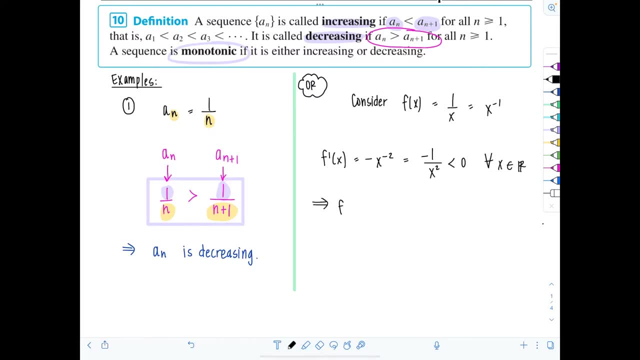 On the real number line. So what does that tell me? That tells me f of x is decreasing on all real numbers, or negative infinity to infinity. And since I've shown that f of x is decreasing, I'm going to take the derivative of x to the negative first, and then I'm going to take the derivative of x, And since I've shown that f of x is decreasing, I'm going to take the derivative of x to the negative first and then I'm going to take the derivative of x to the negative first. So what does that tell me? That this derivative of x is decreasing on all real numbers or negative? 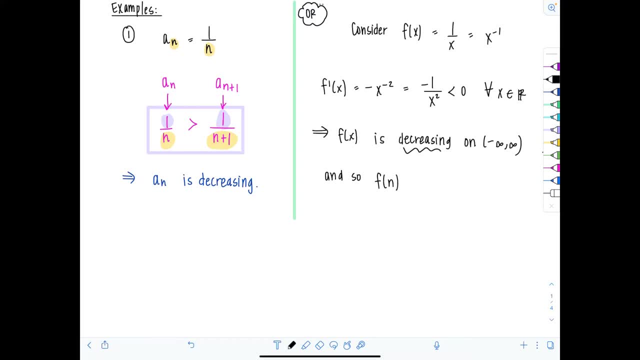 infinity to infinity. This means f of n is going to be greater than f of n plus one, And basically that allows me to now say that the sequence a- n is decreasing. All right, Good, So either way, you can just use the definition directly, like we did here. 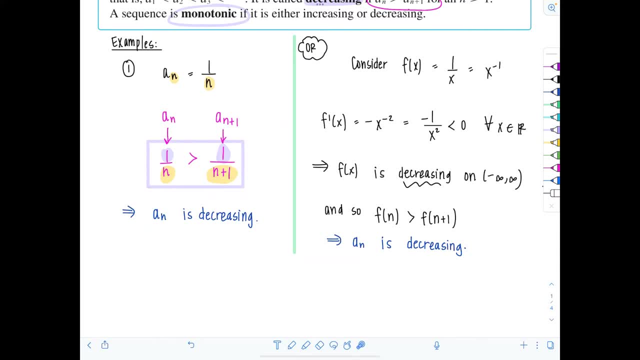 establish an inequality and conclude that the sequence is decreasing. All right, So now I'm going to take the derivative of x to the negative first, and then I'm going to. or you can take a derivative, and as long as you can show the derivative is always negative, or 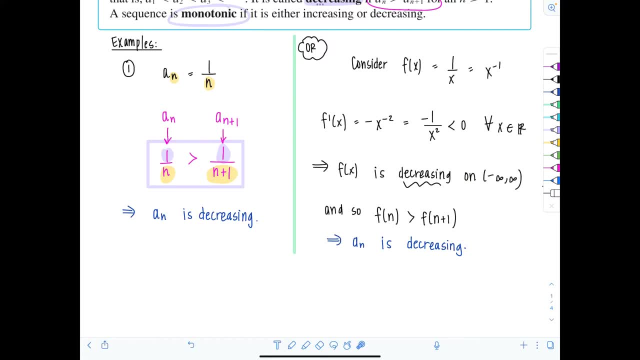 always positive on some interval. then you can say: the sequence is either going to be increasing or decreasing there. What's not okay to do is just list out some terms and say: see they're getting smaller, or see they're getting bigger, Uh-uh. you can't do that. That's not establishing that. 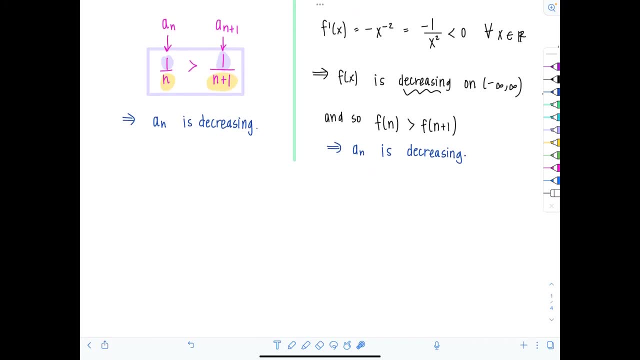 a sequence is increasing or decreasing. It can be helpful if you're not sure right and you want to list out some terms just to get a feel for what's going on. That's not a bad idea if you just don't even know where to start but don't feel like that's going to be sufficient justification in. 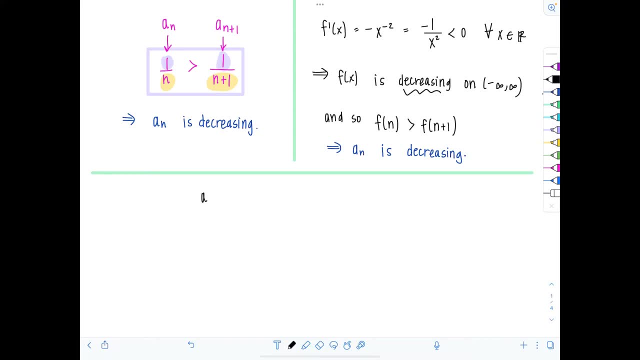 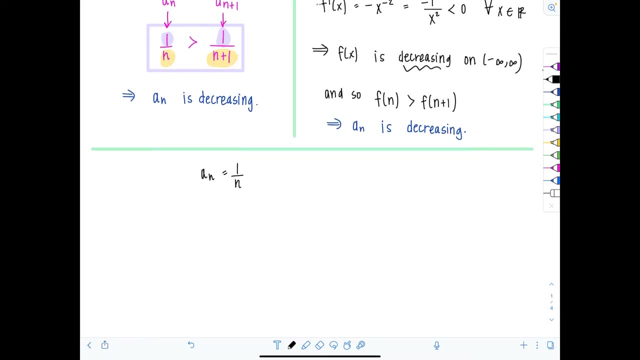 any scenario. okay, Cool. So a n, remember, was 1 over n. Let's list out some of the terms just so you guys can see. So a 1, that would be 1.. a 2, 1.. 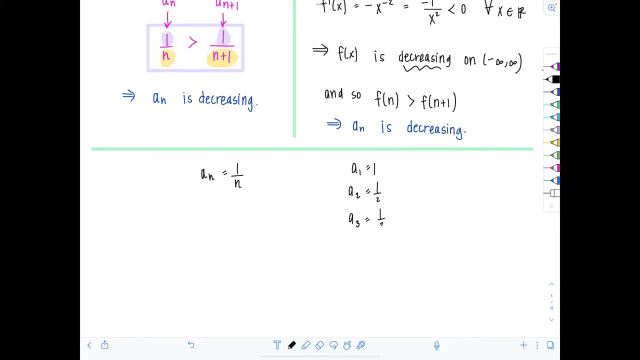 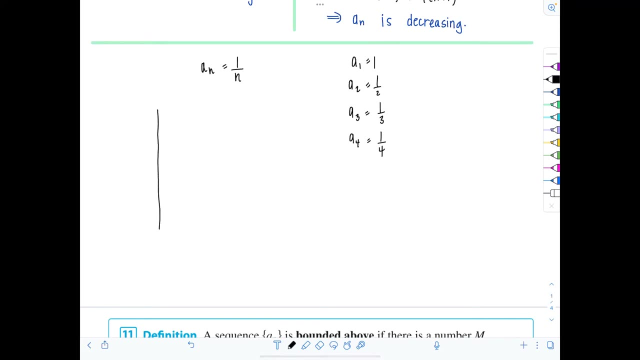 1 1⁄2, a 3, 1 3rd, a 4, and you're probably like: oh yeah, it's so obvious it's decreasing, okay. So when you show it, though, you just have to either use the definition, establish an inequality. 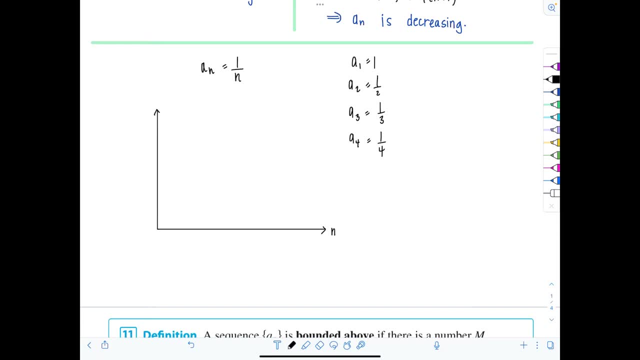 or take a derivative, Let's just plot it for funsies. So here's n, here's a n. 1, 2, 3,, 4, 5, and then it doesn't look like they're going to be larger than 1.. 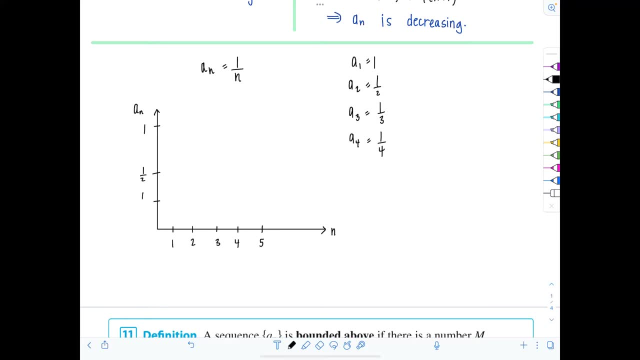 So 1,, this is 1⁄2, this is 1⁄4,, 1⁄8,, et cetera. Let's just plot some of them: a 1 was 1,, a 2 was 1⁄2,, a 3 is 1⁄3,- that would be like right around here- a 4, 1⁄4,, 0.2,, et cetera. okay, 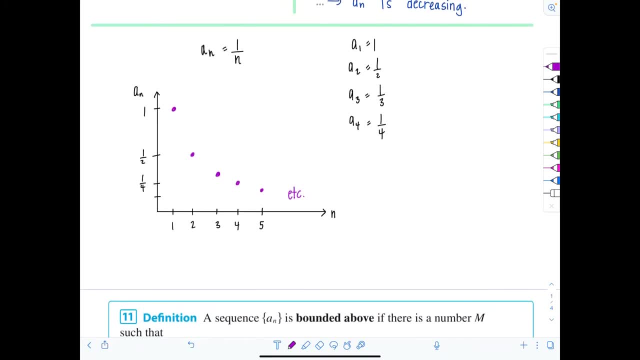 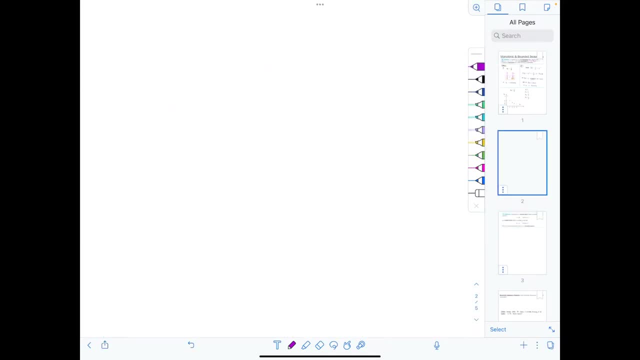 Let's look at another one. Definition popped up too early. Hold on, let me get some space. Okay. another example of a sequence. Let's look at example 2.. a n is equal to cosine of n. Okay, so if you're going to try to compare a n plus 1 with a n, it might be a little tricky in this case. 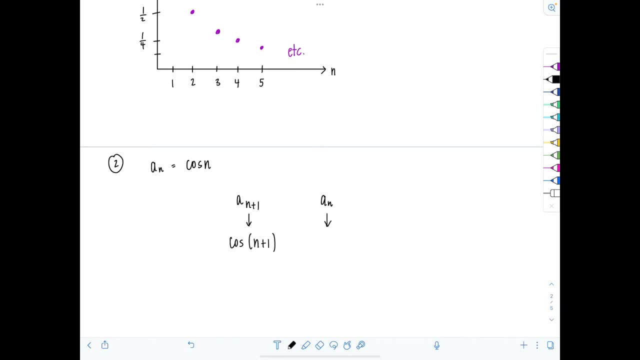 because you have cosine n plus 1.. And then compare it to cosine of n. I don't know necessarily which one's larger or smaller. Remember cosine of x or cosine of n? either way, it's going to have cyclical or repeating values. 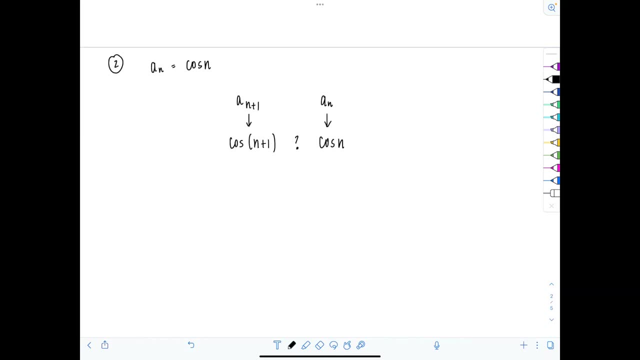 So who's to say which one's larger? Let's start listing out a few terms to get a feel for what's going on, and then we can strategize what we're going to do. So a 1 would be cosine of 1.. 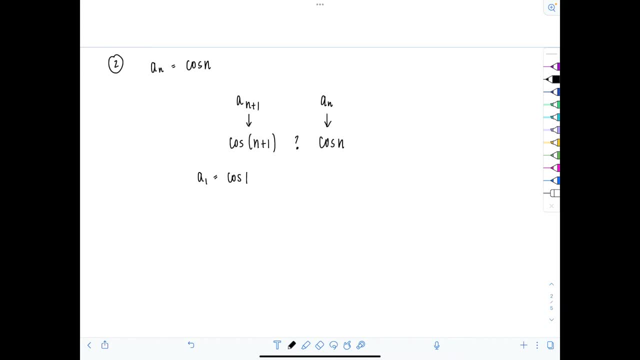 Cosine of 1.. I know it's going to be positive because we're still in quadrant 1.. If you want to get your calculator out just to have some decimal approximation, it's about 0.54.. a- 2,, that would be cosine of 2.. 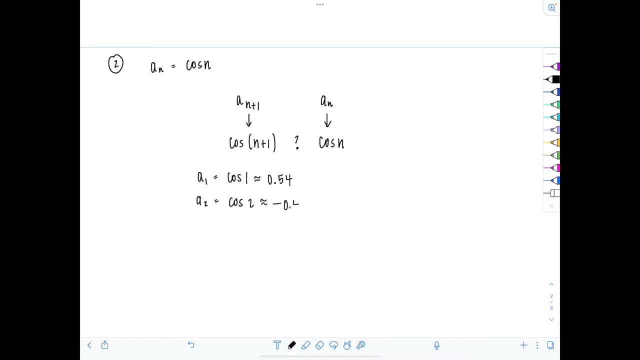 Now I know we're in quadrant 2, so it should be negative and that's negative 0.42.. So maybe at first you think, hmm, it looks like it's decreasing right, It went from positive to negative. Let's see if that keeps up. 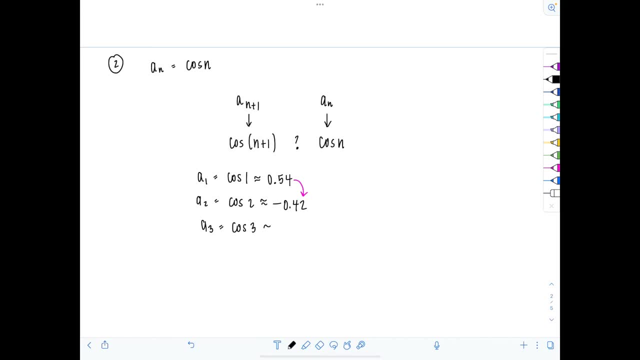 a 3.. That would be cosine of 3,, which is about negative 0.99.. Ooh, it looks like it's still decreasing. But then a 4 is cosine of 4, and that's about negative 0.65. 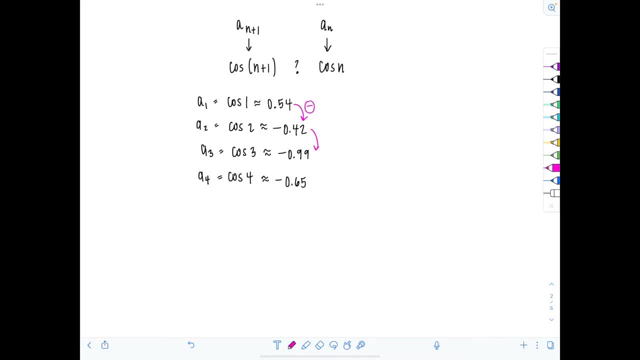 So it was decreasing, then it was decreasing again, and then the sequence increased, And that's enough to just say hey, it's not monotonic. okay, I'm not trying to show that it's increasing or decreasing anymore, so I can just by observation say: check it out. 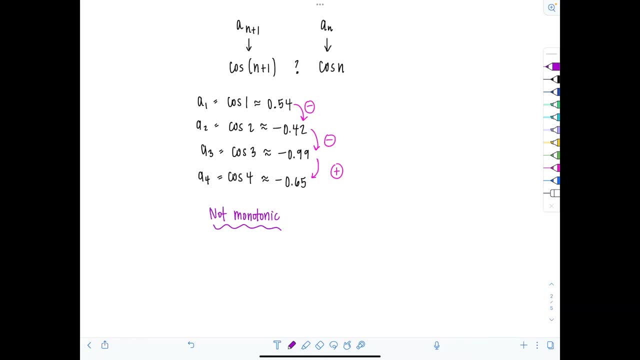 The terms are all over the place. They're going up, they're going down, which we expect. right, It's cosine, come on, It's not monotonic. This sequence increases and decreases, and we are done. Okay, so some sequences can be increasing, some can be decreasing, and then some can be neither. 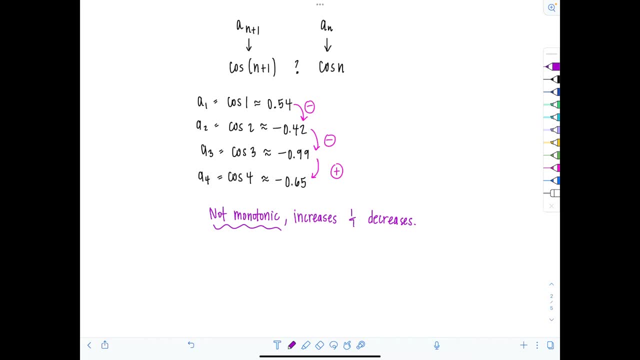 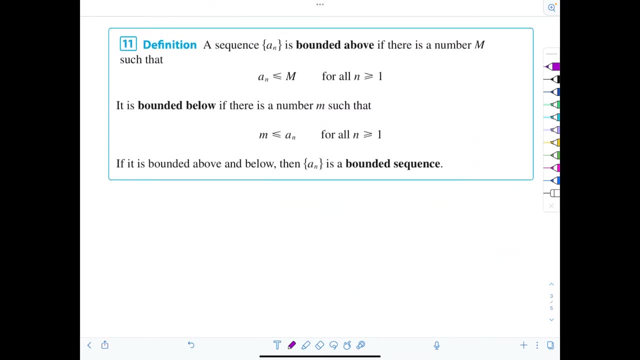 They can just be bouncing all over the place. Now we also want to introduce one other important concept about a sequence, and that is whether or not it's bounded. So a sequence- a- n- is bounded above. if there is a number m such that a- n, all of the terms are less than or equal to m, for all n greater than or equal to 1.. 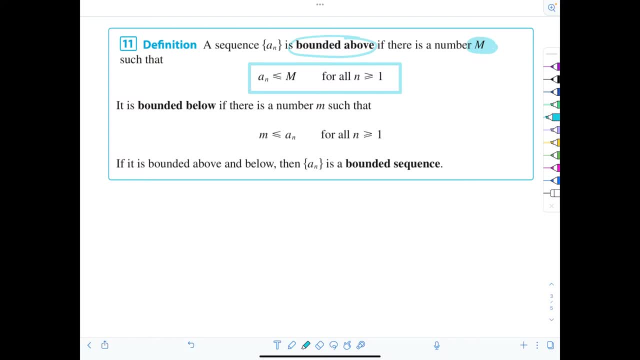 And then we say a sequence is bounded below. if there's a number, Usually we call it lowercase, We call it lowercase m, the lower bound, such that all of the terms a, n are greater than or equal to m. And if a sequence is bounded above and below, so you can find an upper bound and a lower bound, then we say a- n is a bounded sequence. okay. 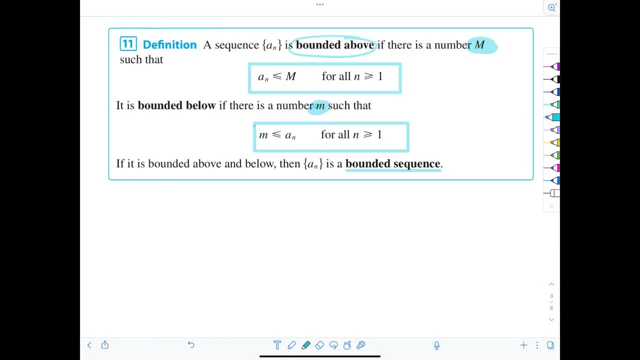 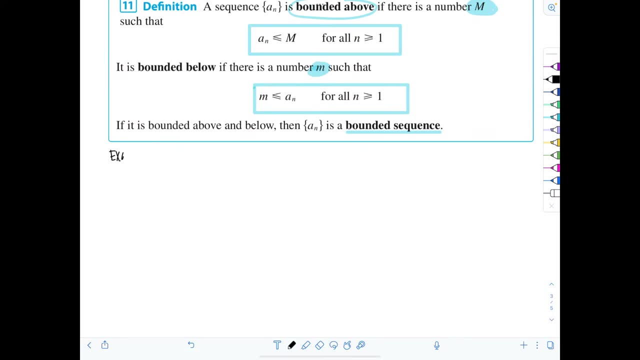 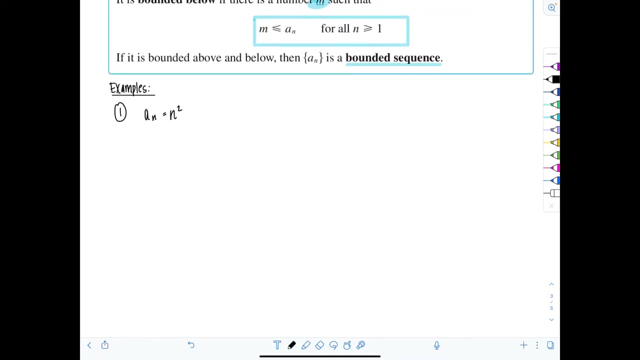 So let's see if we can determine whether or not some sequences here are bounded, and then we'll put this all together. So examples First one: let's look at the sequence a- n, which is n squared, okay. So let's just list out some of the terms to get a feel for what's going on. 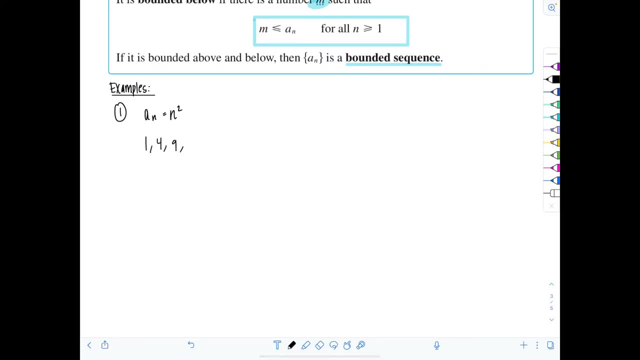 1,, 2 squared is 4,, 3 squared is 9,, 16,, 25,, etc. So it looks like for sure the sequence is bounded below, because the terms appear to be bounded below. So it looks like for sure, the sequence is bounded below because the terms appear to be bounded below. 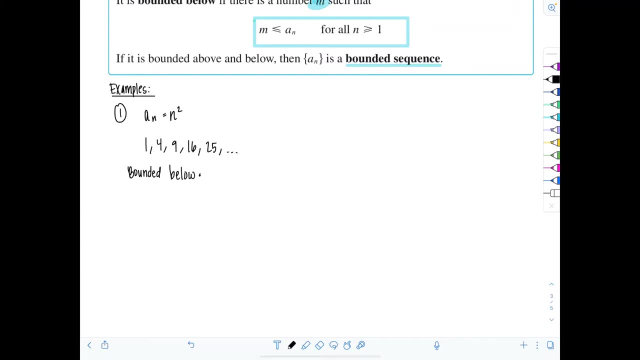 So it looks like for sure the sequence is bounded below because the terms appear to be bounded above. What could I say is a lower bound, So all of the terms have to be greater than or equal to your lower bound. I could say: all of the terms are greater than or equal to 1, so m my lower bound is 1.. 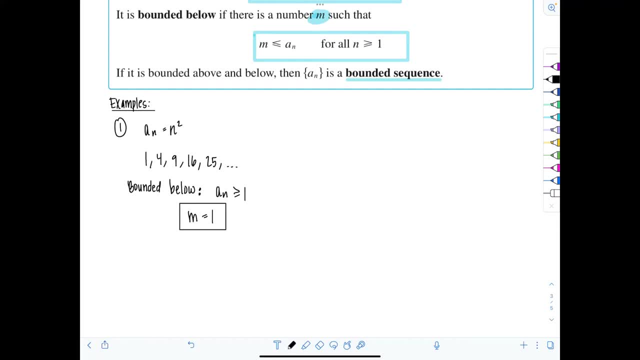 It would also be true if you said m is 0. It is correct that all of the terms are greater than or equal to 0.. Later on in math, you'll study the same thing. Later on in math, you'll study the same thing. 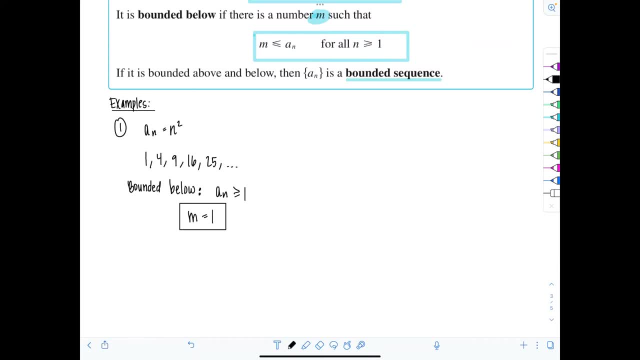 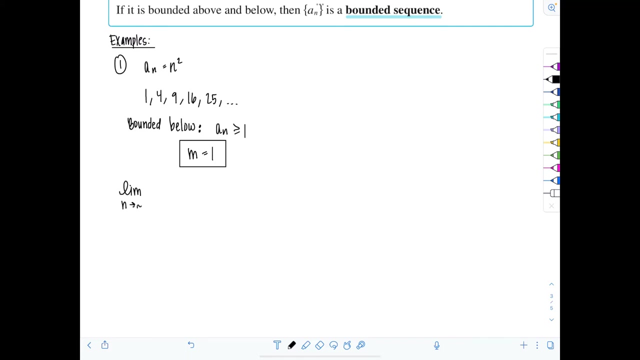 concept of the greatest lower bound, and so you want to try to get as close as possible, basically, to the threshold of the terms when you're determining a lower bound. okay, so the sequence is bounded below: can we figure out an upper bound? hmm well, let's look what happens as n approaches infinity to the terms. 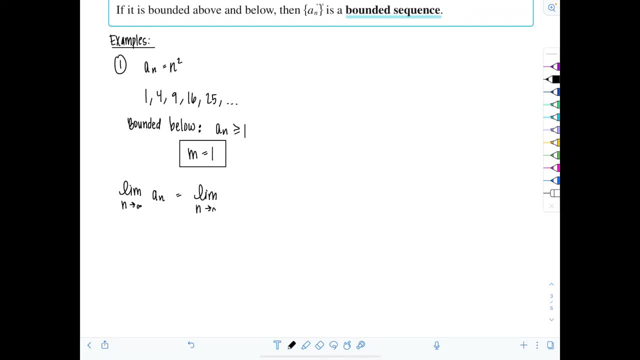 what is the limit? as n approaches infinity of n squared, it just goes to infinity right. so that means the sequence is not bounded above. and remember, for a sequence to be considered bounded you need to find both an upper bound and a lower bound. so that tells us a n is not bounded. 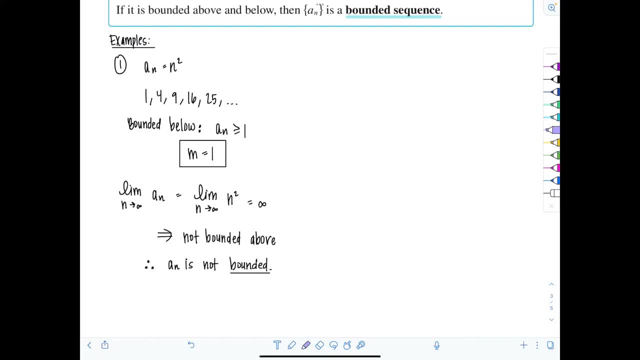 okay, let's look at another case, another sequence, example two: oh, how about that cute little cosine of n? well, you should remember from trigonometry, cosine is always bounded between one and negative one. so this sequence is most definitely bounded: my upper bound is one, capital M, and my lower bound, negative one, is: 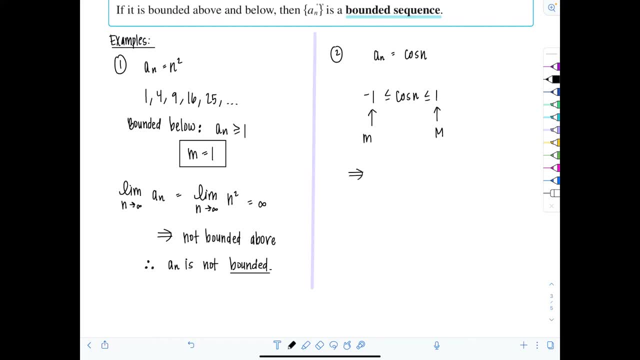 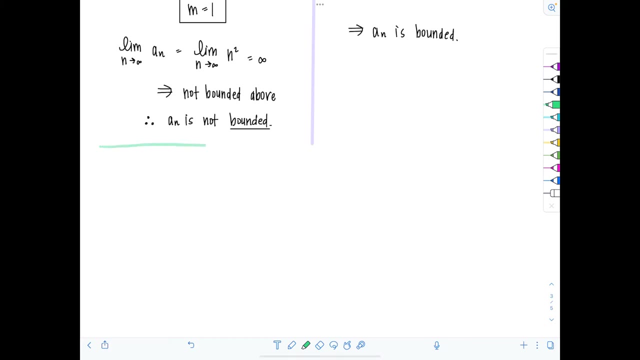 lowercase M, and that's really all there is to it. this should just be an inequality of fact that you have ready to go and is therefore bounded. all right, let's just check out one more. do you remember that very first sequence we looked at, a n is one over N. yeah, well, remember. the first term would just be. 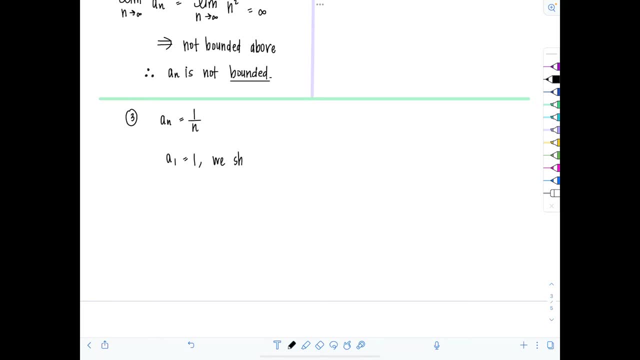 one over n and negative, one over n is just that, and so right, therefore, we are bound. and then what's the first equation when we set the over 1, which is 1, and we showed earlier that an is decreasing. so if the sequence is decreasing, that means its first term is the largest value that it's ever. 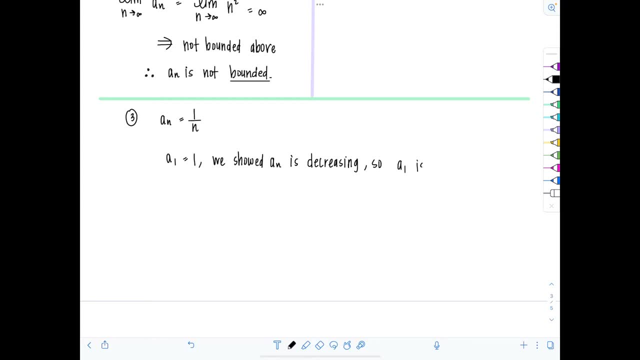 going to take on. so that tells us that a 1 is an upper bound. right, if the sequence is decreasing, an upper bound, the largest it's ever going to be, is that first term? so I could say: capital M, my upper bound is 1. now can I find a? 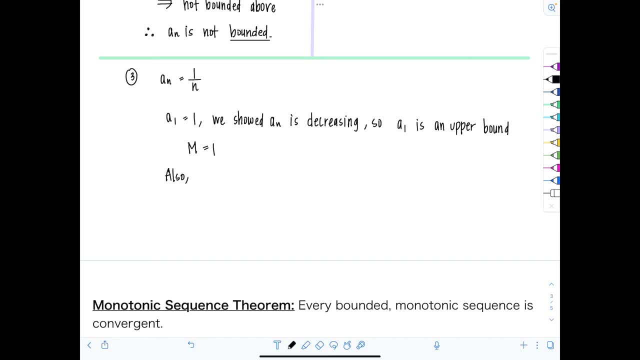 lower bound. well, let's consider what happens as n gets bigger. so, to do that, we're gonna take the limit, as n approaches infinity, of 1 over n, and this is 0. so what does that tell me? well, the terms aren't ever gonna go to negative. 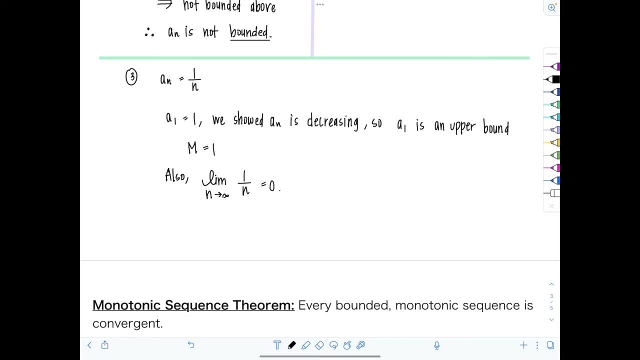 infinity or blow up somewhere else. so in fact, I also know that the terms are never even gonna be negative. all of them are greater than or equal to 0, right for all n greater than 1 or equal to. so what can I say? I could say an is. 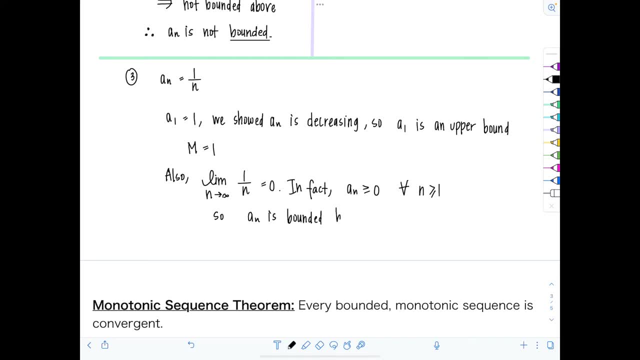 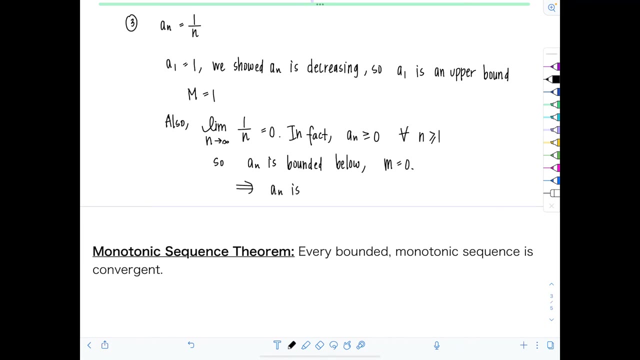 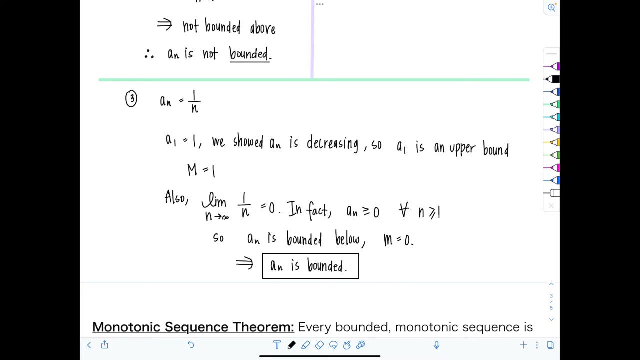 bounded below, and its lower bound is 0, so all of the terms are going to be greater than 0. therefore, what can we say? we found both an upper bound and a lower bound, so So AN is bounded, And so usually you'll answer both questions about a sequence together, whether or not it's monotonic and whether or not it is bounded. 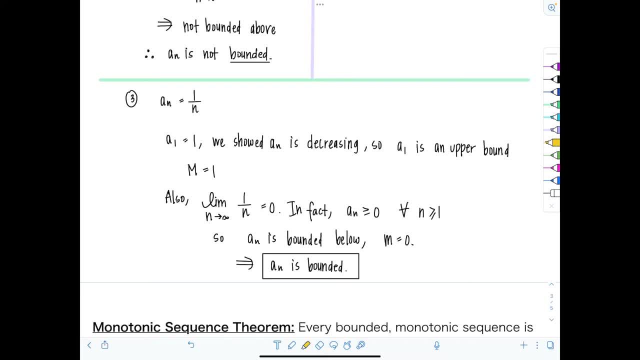 And knowing that a sequence is monotonic, just like we knew that this sequence was decreasing, helped us find the upper bound right. But also, putting these two characteristics together leads us to an important theorem, And it's the monotonic sequence theorem. 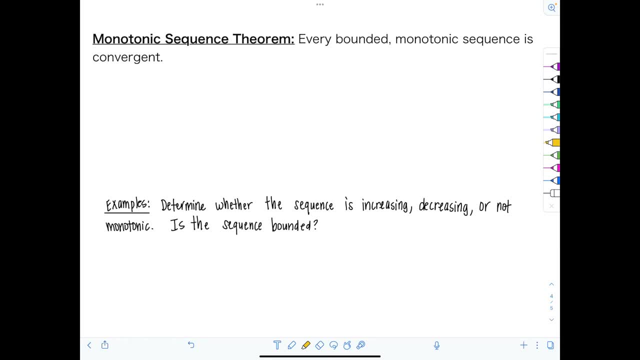 It says: every bounded, monotonic sequence is convergent. And this is a big deal, because sometimes it's very difficult to establish convergence for a sequence. But if you can establish that it is monotonic and bounded, then bam, you bust out the theorem and you go. we know it's convergent. 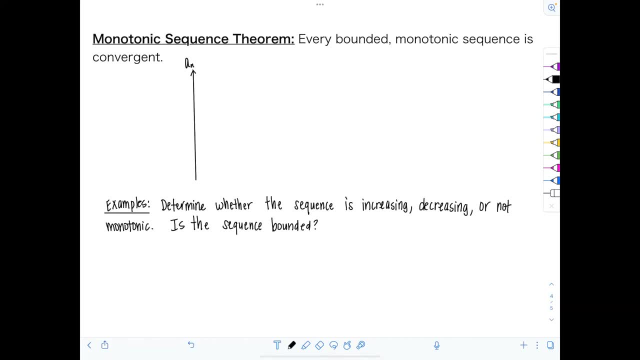 And I want you guys to understand this. So let's graph A few arbitrary sequences just so you can understand why this theorem should make sense. So every bounded monotonic sequence is convergent. If it's bounded, then that means there's an upper bound and a lower bound that all of the terms live between. 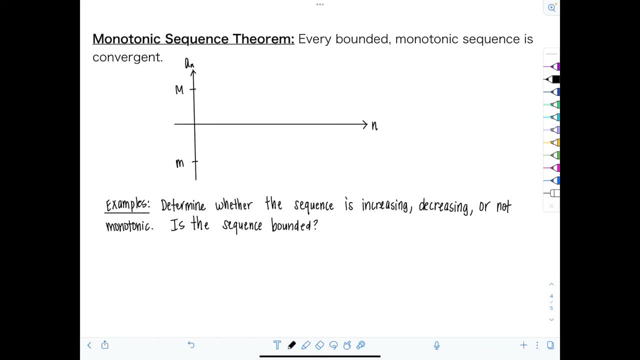 One doesn't have to be positive and the other one has to be negative. Just, capital M is bigger than lowercase m. Good, So here's the upper bound, Here's the lower bound, And they're telling us. the sequence is monotonic. 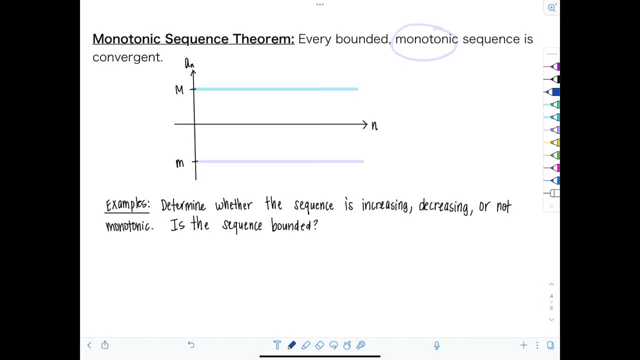 So if the sequence is going to be monotonic, that means all of the terms are either going to be decreasing, getting smaller, or the terms of the sequence are going to make it increasing. They're just going to be getting bigger And you can see if the sequence is always getting bigger. 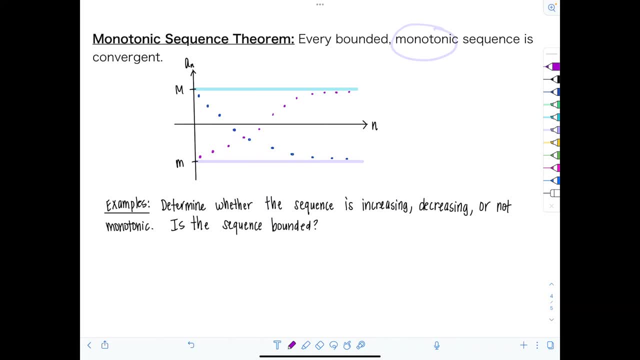 or the terms are always getting smaller and the terms are trapped between an upper bound and a lower bound. eventually they approach a limit, The terms converge, So that helps us establish that the sequence is convergent. See, your sequence is not monotonic, even though it's bounded. 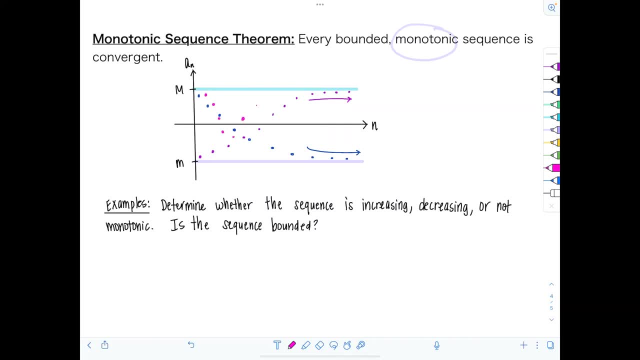 So it can decrease, and then maybe it's going to increase, and then it's going to decrease, and then it's going to increase, much like cosine did, right? So in that case, no, the sequence is not convergent. 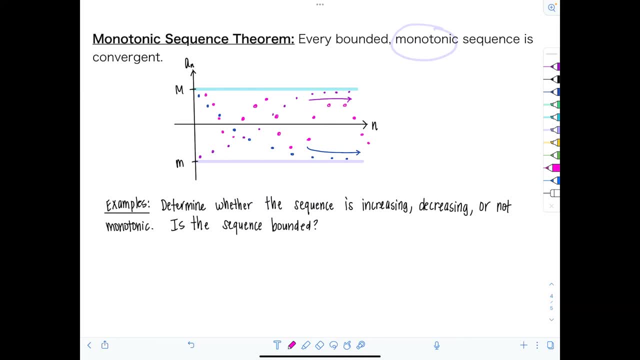 The terms don't approach some constant, even though it's bounded. So you see why both are necessary, both conditions, And that's very important if you're going to study more math down the road, hopefully. So let's answer this question now. 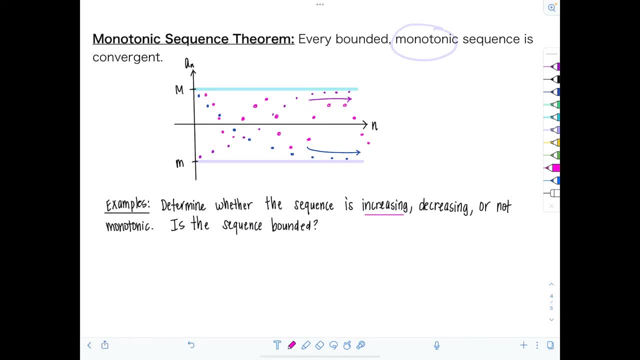 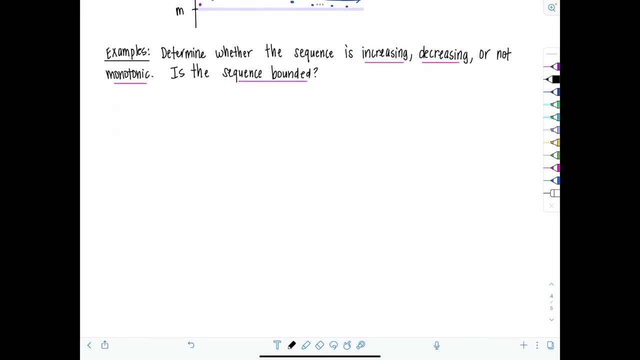 Determine whether the sequence is increasing, decreasing or not monotonic. That's possible. And then, second part of the question is the sequence bounded. All right, Here we go. I got four lovely little examples for you. Example one: 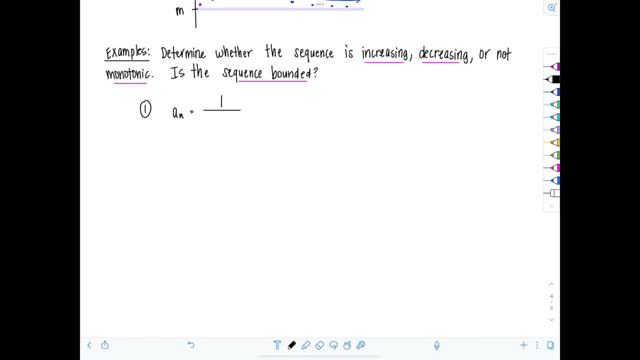 The sequence a- n is 1 over 2n plus 3.. Okay, So let's just see if we can use the definition to establish whether or not the sequence is increasing or decreasing. So let's look at what a n plus 1 is. 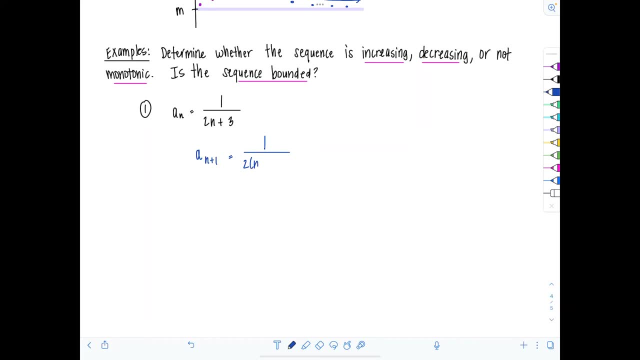 a n plus 1 would be 1 over 2 times n plus 1 plus 3.. Right, And then if I distribute and clean up, this is 1 over 2n plus 5.. So now compare it to a n. 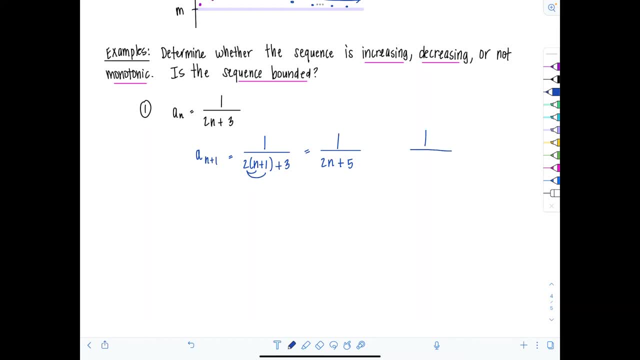 a n was just 1 over. let me do it down here. so 1 over 2n plus 5, compared to a n which is 1 over 2n plus 3.. Is it clear that one is always larger than the other? 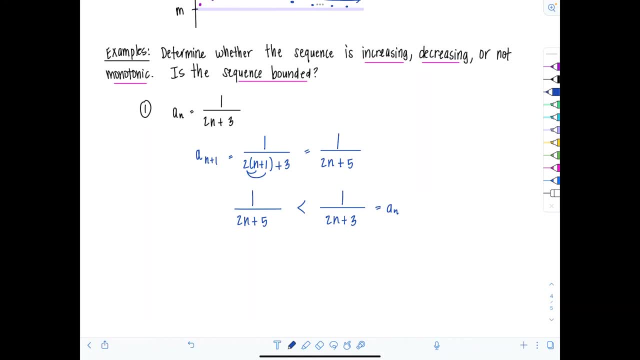 Yeah, for sure I can see that a n is always going to be greater than a n plus 1.. So what does that mean? That means the terms are getting smaller, so a n is decreasing. Bam, We've answered the first question. 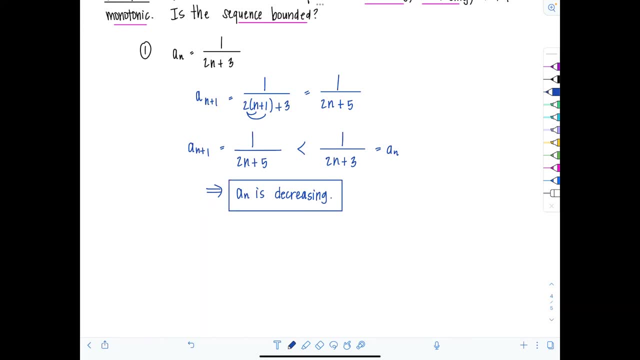 The sequence is decreasing. Now is it bounded, So I know the terms are getting smaller. okay, That means a 1 is going to be an upper bound, So we can say a 1, what would a 1 be? It would be 1 over 2 plus 3.. 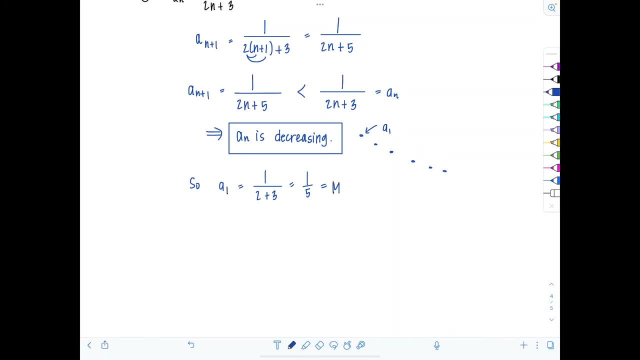 That's 1 fifth. I'll call that capital M. That is an upper bound. Now do we have a lower bound? When you know the sequence is decreasing and you have an upper bound already established, you want to go ahead. 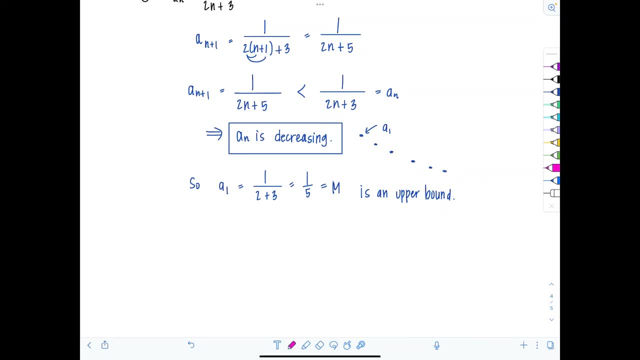 take the limit as n goes to infinity. Why? Because I want to know: are the terms going to level off, or do they just keep decreasing forever, without bound towards negative infinity, perhaps? All right. So that's a typical step. Once you've already established, your sequence is monotonic. 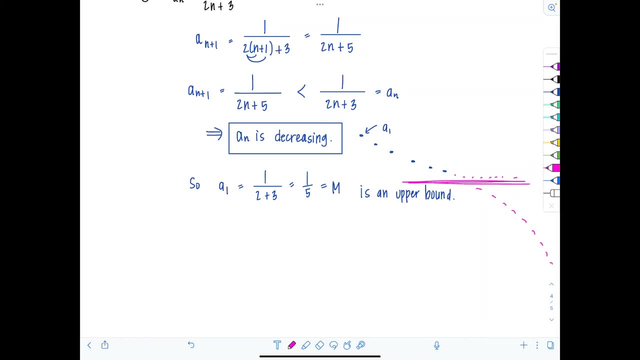 and you have either the upper bound or the lower bound. take the limit as n approaches infinity. So let's see the limit as n approaches infinity of 1 over 2n plus 3.. Yeah, I can clearly see that is 0,. 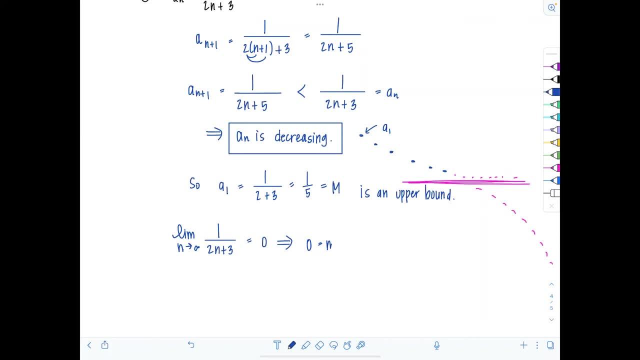 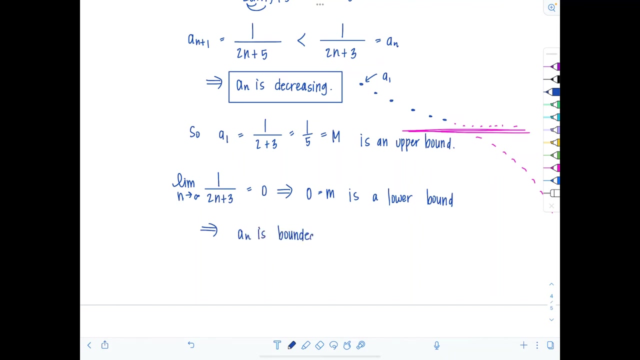 which means 0 can be my lower case, m, That is a lower bound. Therefore, an is bounded. And that was all the you know the directions asked us for. Is the sequence monotonic? Is it bounded? We can also say: 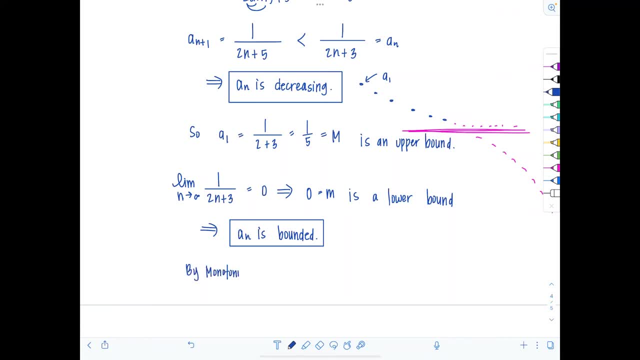 by the monotonic sequence theorem. this means that an is convergent, But they didn't ask us: Whatever We're ready. We're ready for whatever comes our way. Okay, Good, Let's look at some more examples. Don't you fret? 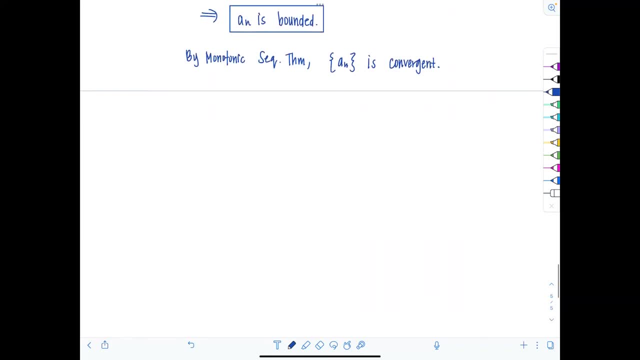 This is going to take a little bit of practice. Let's look at another sequence A little more spicy: An, which is equal to 1 minus n over 2 plus n. So sometimes it's nice just to, instead of working with an inequality. 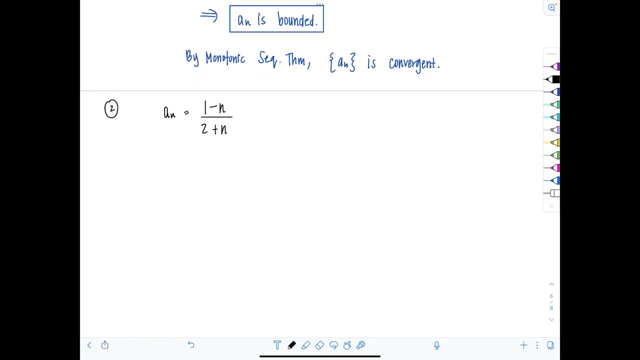 consider a function defined similarly to our sequence And look at its derivative instead. So why don't we go ahead and try that with this example, Just because it looks a little more complicated? So let's consider f of x, which is equal to 1 minus x, over 2 plus x. 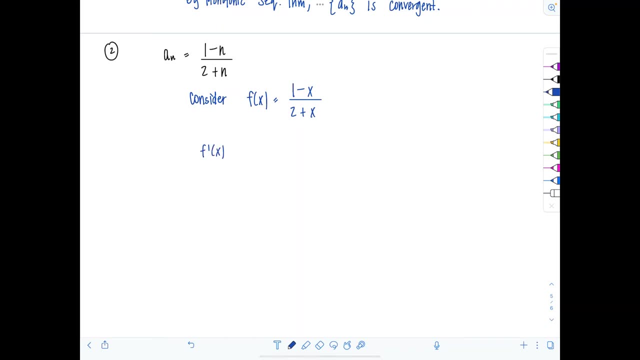 So I want to look at the derivative of this function And I need to apply the quotient rule. Yeah, Do you remember the quotient rule? I always sing this little song: Low d high. so denominator times: derivative of the numerator minus high. 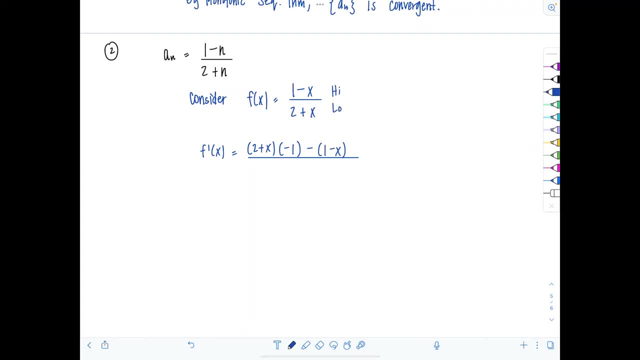 that means the numerator d, low derivative of the denominator Square the bottom away you go. Okay, Time to distribute. So this is negative: 2 minus x, minus 1 plus x over 2 plus x squared And notice: 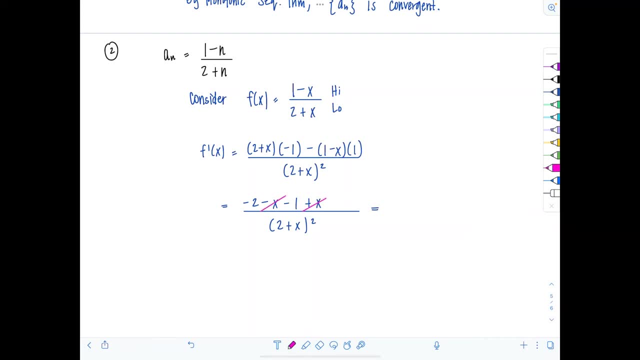 x will cancel out here. So we've got negative 3 over 2 plus x squared. Ooh, this is good. This is good because I've got a negative 3 in the numerator And then notice the denominator has a quantity squared. 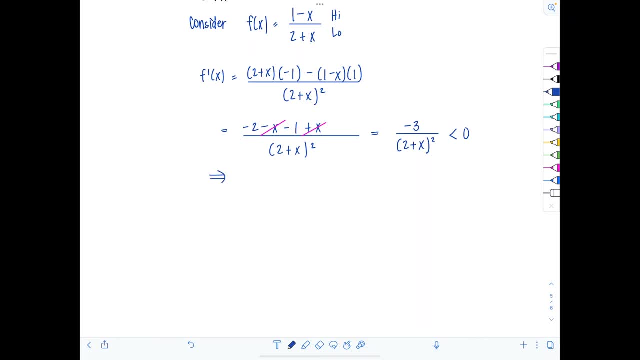 So for sure, this derivative is always less than 0. That means f of x is decreasing. So you could say: f of n plus 1 is going to be less than f of n And that means a n, our sequence, which is 1 minus n over 2 plus n. 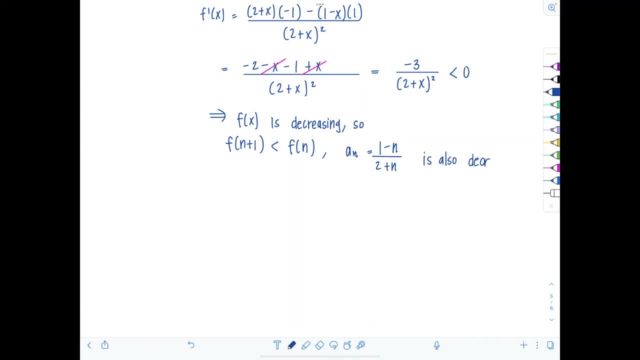 is also decreasing, All right. So if it's decreasing, the terms are going like this: That means automatically, I know an upper bound is going to be the first term, which is a 1.. So a 1 would be 1 minus 1 over 2 plus 1.. 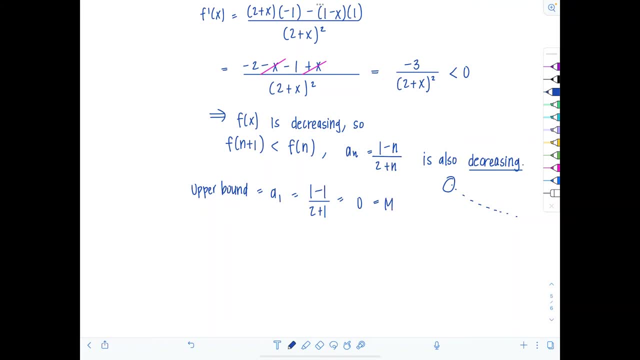 That's 0 over 3, which is 0.. So there's my upper bound. Good, Now what question do I have to answer? Is there a lower bound? How can we do that? Think back to the last example. 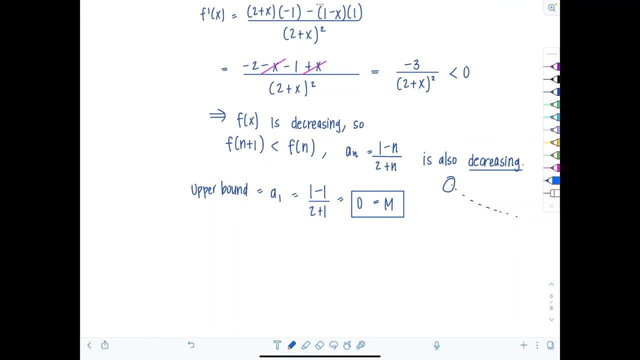 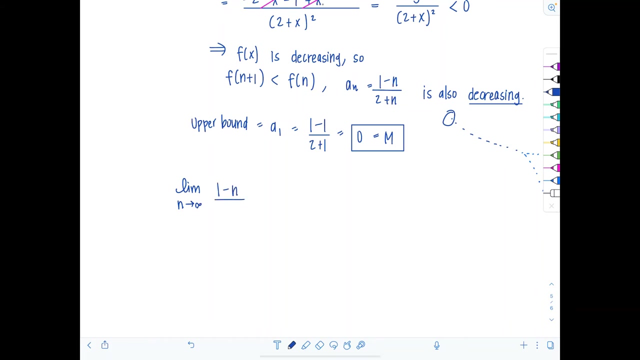 I want to take the limit as n goes to infinity to see: do the terms level off or do they just go down forever, keep decreasing without limit, right? So now we're going to look at the limit, as n approaches infinity, of 1 minus n. 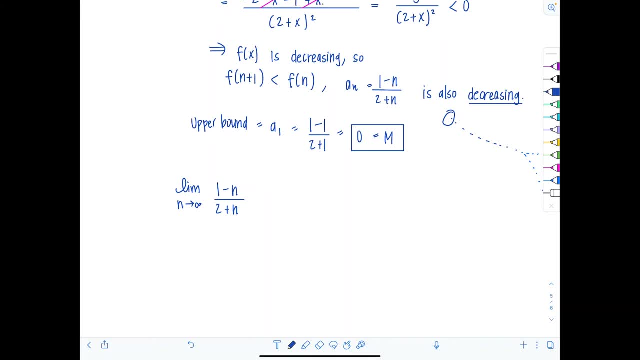 over 2 plus n. So to take this limit, I'm just going to divide by the highest power of n in the denominator, which is the same as multiplying by 1 over n top and bottom, And let's see what we have when I distribute that through. 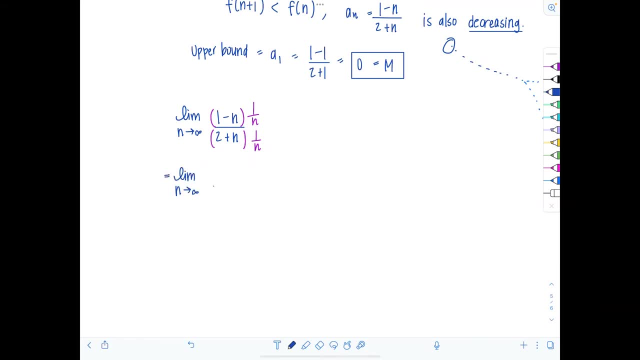 So this is going to be the limit: n approaches infinity. In the numerator we're going to have 1 over n minus 1.. And then in the denominator, 2 over n plus 1.. And then, as n goes to infinity. 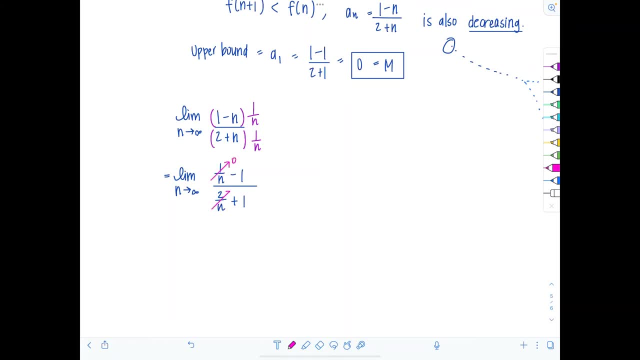 it's clear: 1 over n will approach 0.. 2 over n will approach 0.. So all I'm left with is negative 1 over 1.. And that is negative 1.. So what does that tell me? That tells me: the terms don't decrease without limit. 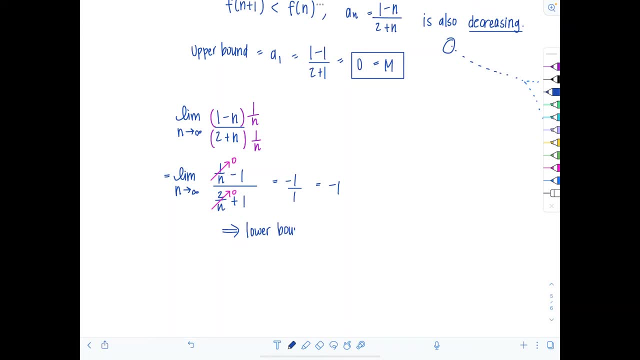 that in fact we have a lower bound, negative 1. So that's lowercase m? Great, Great, great great, I found an upper bound, I found a lower bound. So what does that tell me? It tells me that my sequence: 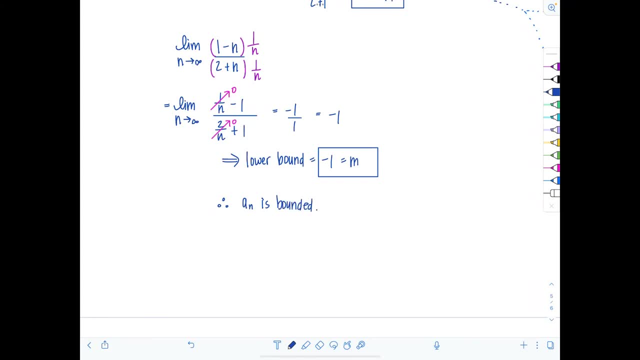 a? n is indeed bounded. You could always add to by the monotonic sequence theorem. we know that a? n is also convergent if they ask: All right, how are we doing? Getting the hang of it a little bit. 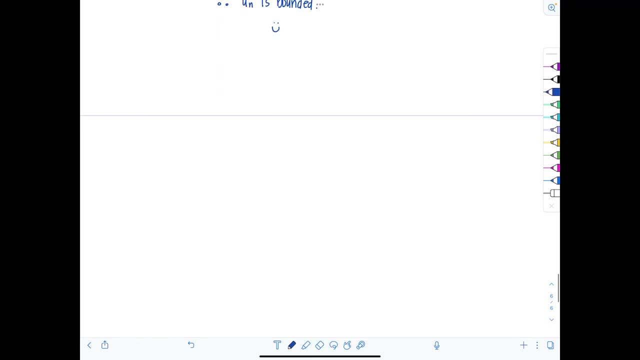 Yeah, Okay, Let's check out some other scenarios that can come up. So example 3, a n is n cubed minus 3n plus 3.. Hmm, all right, I don't really feel like figuring out an expression for a n plus 1,. 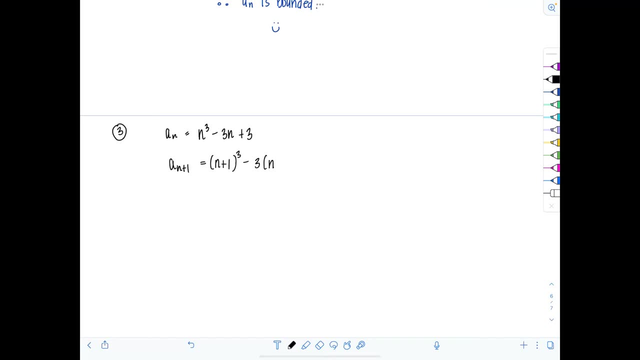 because then I'm going to have to cube this. Oh my goodness, It might be a mess. So instead of doing that, let's just consider a function f of x, which is equal to x cubed minus 3x plus 3,. 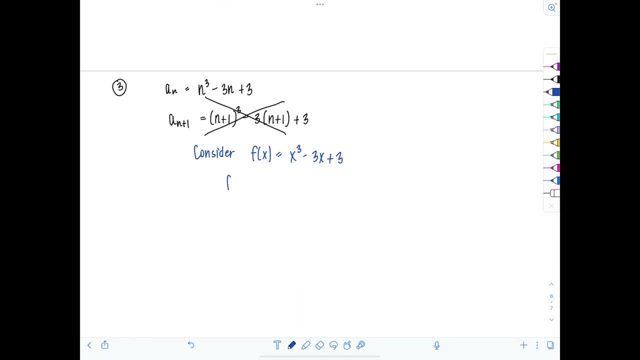 and see if we can look at its derivative. Ooh, I like this better. So f prime of x would be 3x squared minus 3.. If I factor out a 3,, I'm left with x squared minus 1, right. 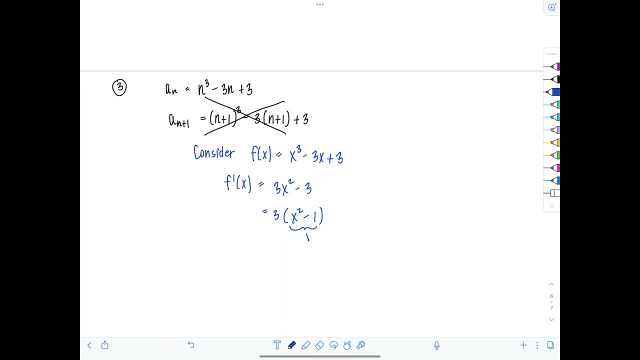 And x squared minus 1, that is going to be greater than 0, as long as x is greater than 1.. And that's perfect for us because, remember, a n is a sequence and usually we don't start plugging in values of n that are less than 1.. 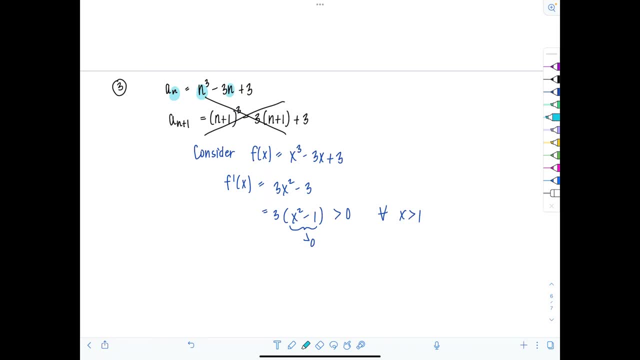 Once in a while you'll plug in like a 0 or a negative 1 if you're told to, but this is perfect that I can show. the function is increasing for all x's greater than 1, and therefore my sequence will also be increasing. 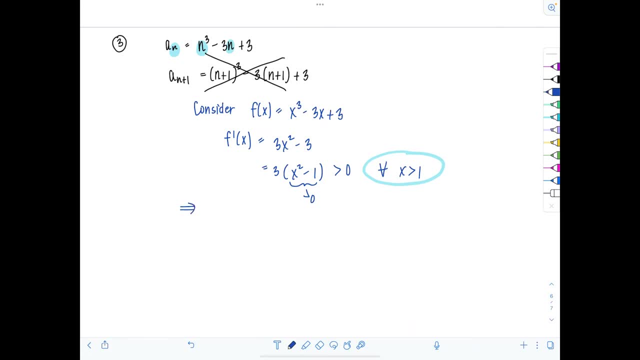 on the same set. So let's summarize it nicely. This means f of x is increasing on the interval from 1 to infinity. Therefore, a n is increasing. Okay, so it's monotonic. However, is it bounded? That's the big question. 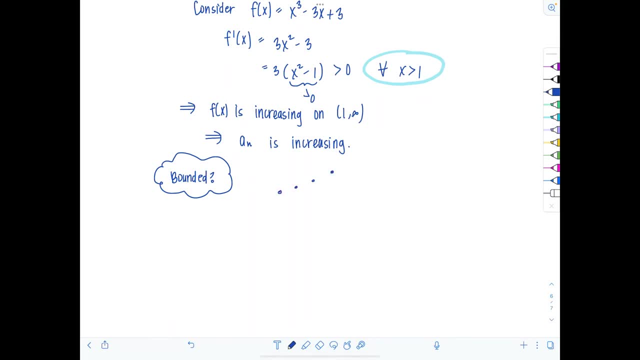 Well, I know my sequence is increasing, so the terms are going like this: up, up, up, up up. Therefore, a 1 is a lower bound. That should be clear. So a 1, where's a n? 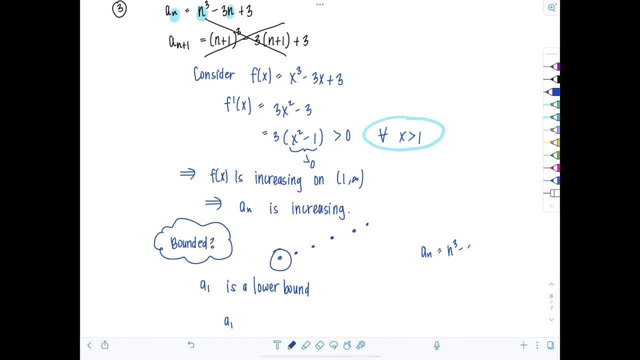 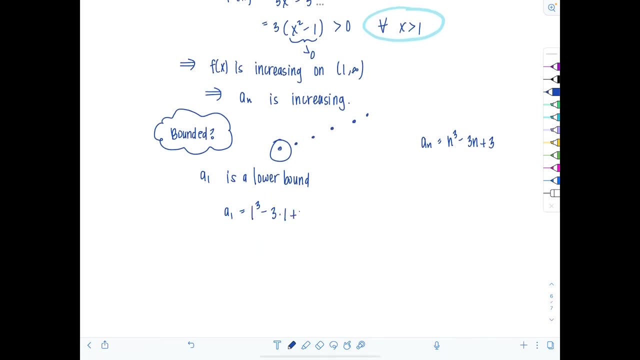 Let's rewrite it here: a n is n cubed minus 3n plus 3.. So a 1 would be 1 cubed minus 3 times 1 plus 3, plus 3. These 3s cancel, So a 1 is just 1.. 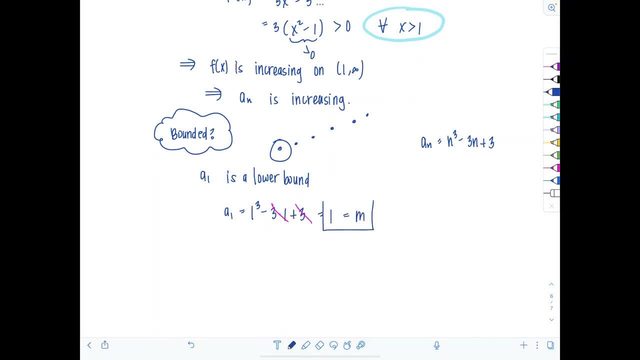 That's a lower bound, so we'll call that lowercase m. Can I find an upper bound? Well, I know the terms are increasing. Do they keep going up forever, or do they level off at some point? How can I answer that question? 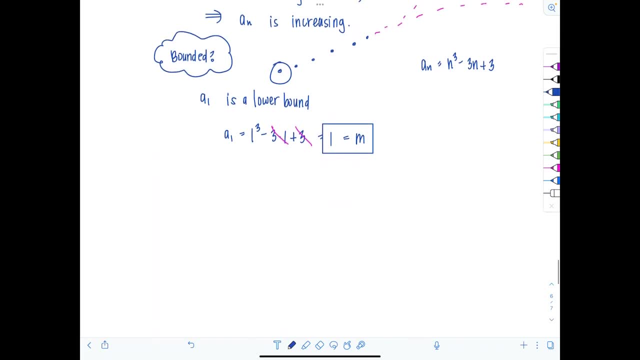 You're going to take a limit. Okay. So the limit as n approaches infinity, of a n, which is n cubed minus 3n plus 3.. Remember when you're taking the limit of a polynomial. Maybe it's been so long, huh. 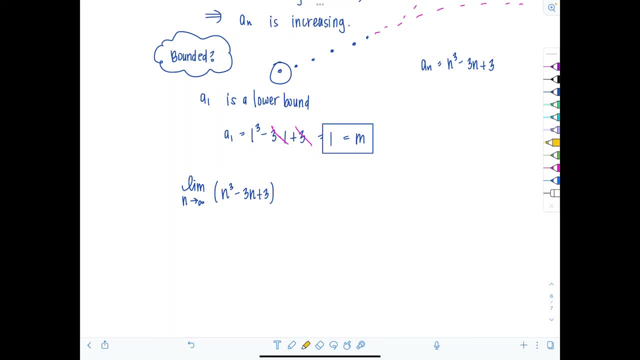 You were just a Calc 1 baby back then. You look at just the highest degree term. So as n approaches infinity, this sequence or these terms will approach positive infinity, which means there is no upper bound. Nope, So the sequence is not bounded. 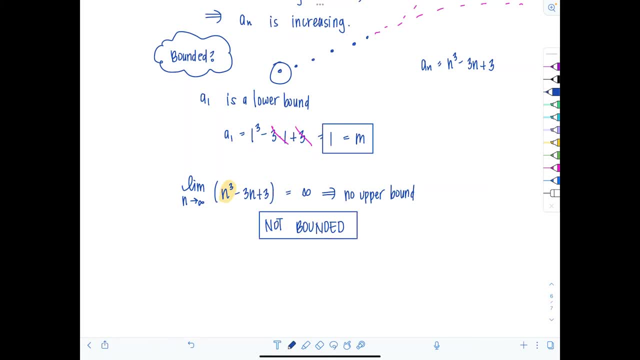 All right, You ready for one more? Last one. Look at that. Are you having fun? I hope so. Example 4 is the grand finale. Here we go. So this sequence is defined as follows: a n is equal to 2 plus negative 1 to the n over n. 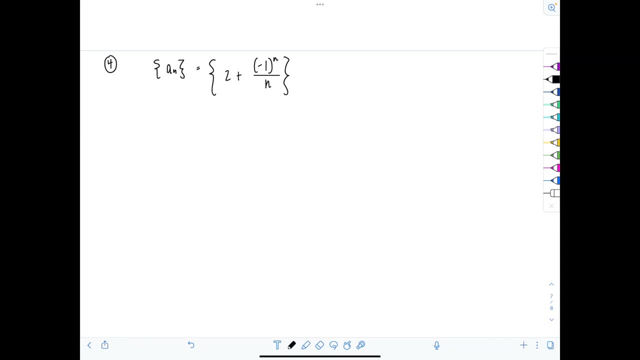 So the sequence is alternating right because of that negative 1 to the n expression. Let's list out the first few terms, just so you can see what's going on. So a 1 would be 2 plus negative 1 to the first over 1.. 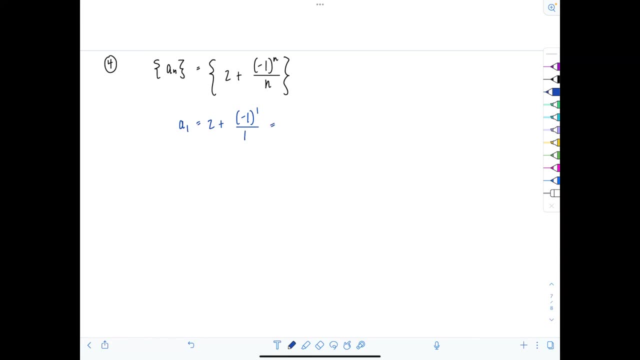 That's just going to be 2 minus 1.. So that's 1.. a 2 would be 2 plus negative 1 squared over 2.. So that's 2 plus 1 half, which is 5 halves. a 3 would be 2 plus negative 1, cubed over 3.. 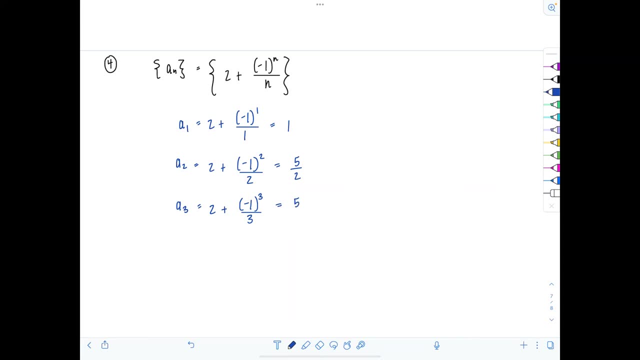 So that's 2 minus 1 third, which is 5 thirds. And already I can see this guy is not monotonic, Monotonic. No, it is not. How do I conclude that so quickly? Well, from 1 to 5, halves the terms increased. 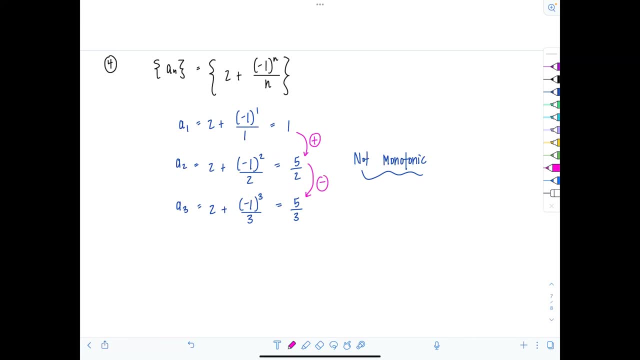 But then from 5 halves to 5 thirds they decreased, And it's just going to keep doing the same thing. If you want to find a 4, why not? It's going to be 2 plus negative 1 to the fourth over 4.. 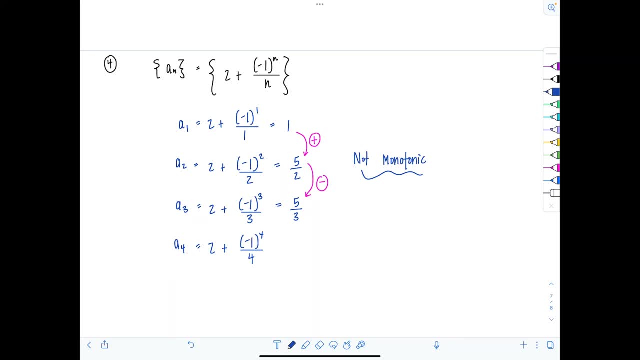 So 2 plus 1 fourth, That's 8 over 4 plus 1 over 4, which is 9 fourths, etc. Now, just because the sequence is not monotonic, the terms increase and decrease, doesn't mean that it's not bounded perhaps. 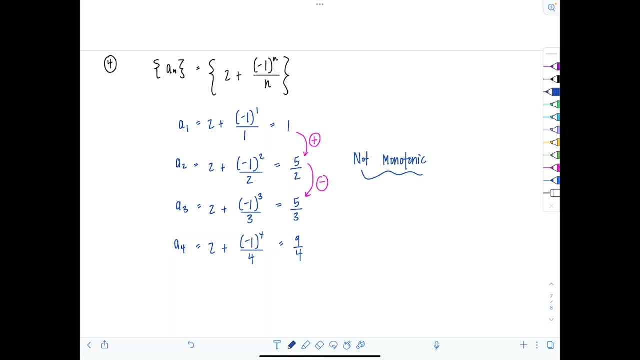 So how can we figure this out? It's really difficult to take a limit, as n approaches infinity, when you have a sequence that's alternating here And typically one thing you can do is figure out where the even terms are going, how they're behaving. 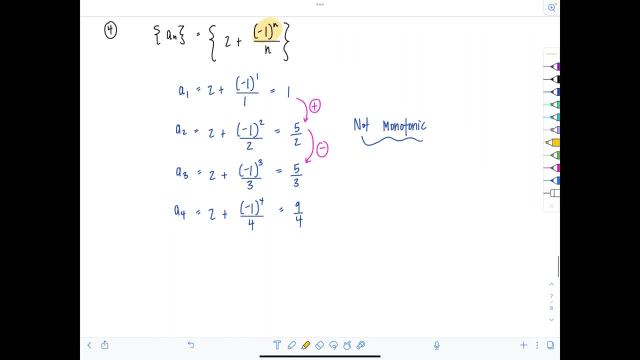 and compare that to what the odd terms are doing. So I'll run you through step by step exactly how to do this. The sequence a n, just to remind you, was 2 plus negative 1 to the n over n. 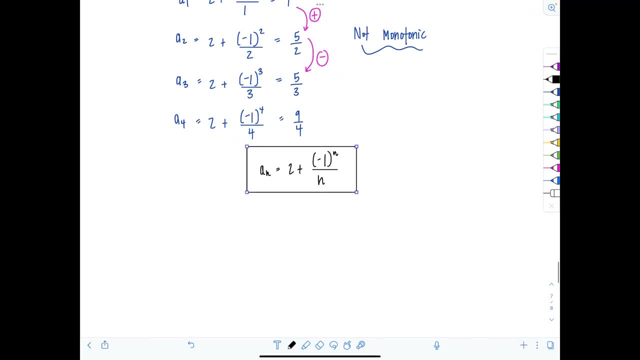 Okay, First let's just analyze what's going on with the even terms. The even terms: When I just want to consider the even terms, I'm going to look at a sub 2 n, And this should make sense. 2 n would generate all of the even terms in the sequence. 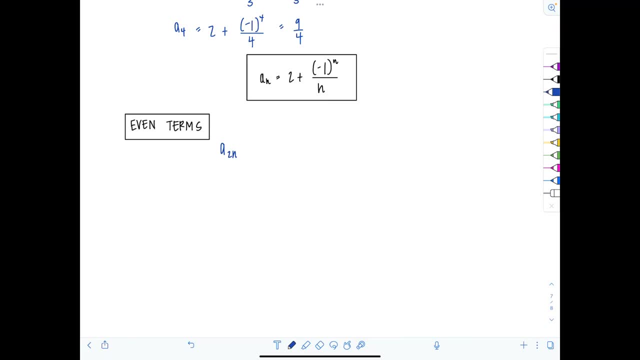 a sub 2,, 4,, 6,, 8, etc. So what's an expression for all the even terms? It would be 2 plus negative 1 to the 2 n over 2 n, And then I can clean this up a little bit. 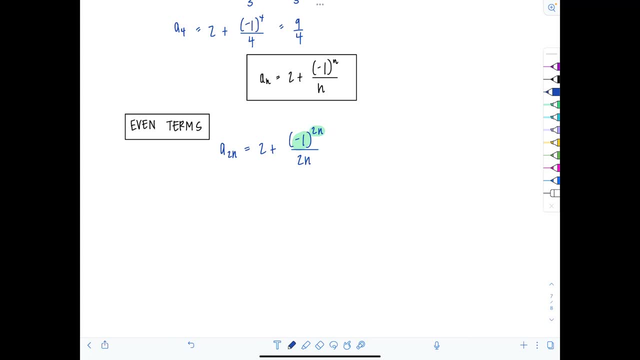 because negative 1 raised to an even power is just going to be positive 1.. So then I could say: okay, a sub 2 n is going to be 2 plus 1 over 2 n. All right, Can I figure out an upper bound or a lower bound? 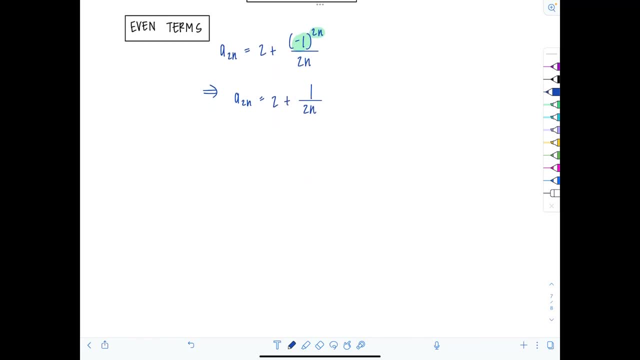 on just the even terms. It's a subsequence. It would help to know if it's increasing or decreasing for sure. So let's consider a function which is equal to 2 plus 1 over 2 x, So we can look at its derivative. 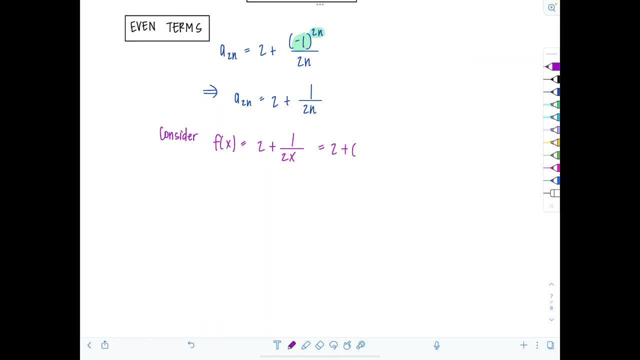 And remember I can write this as 2 plus 2 x to the negative first. So f prime of x, the derivative of 2 is just 0.. And then the derivative of 2 x to the negative first would be negative 2 x to the negative second times 2.. 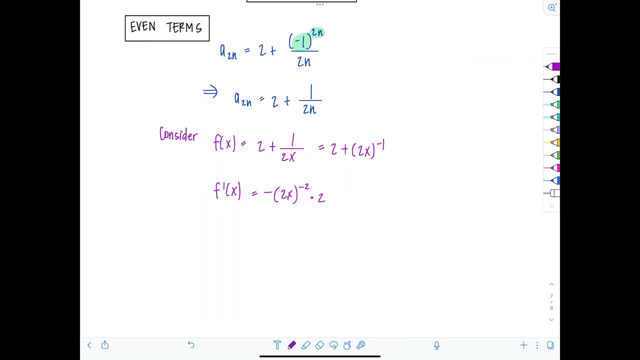 Don't forget that chain rule. And let's see here: This would be negative 2 over 2 x squared. I could clean it up if I want to or not. I can already tell this derivative is always negative. So that tells me the function f of x is decreasing. 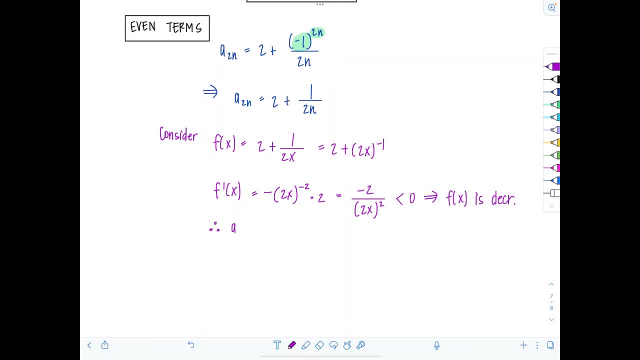 Ooh, that's exciting, because then that means my subsequence of even terms is also decreasing. So if the even terms are decreasing, then that means we do have an upper bound on the even terms. It would be the first even term, right? 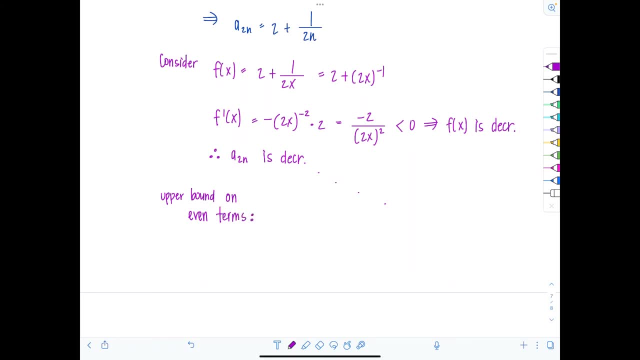 What's the first even term? You guys? a sub 2.. And we already found a sub 2 earlier. It was 5 halves. Okay, So this is an upper bound, but just on the even terms. So I'm not calling it capital M, you know. 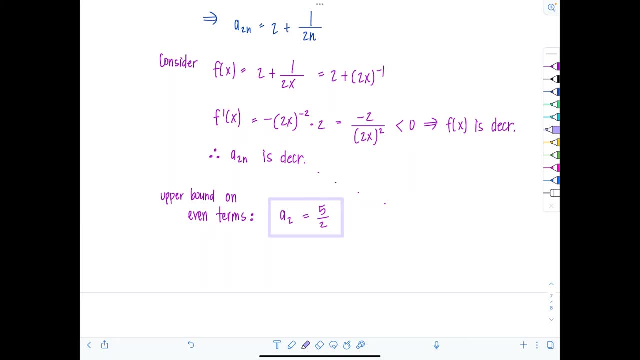 because we want to save that for the whole sequence. Can we find a lower bound on the even terms? Well, the even terms are decreasing. Do they decrease without bound? Do they keep going smaller and smaller and smaller forever, or do they level off? 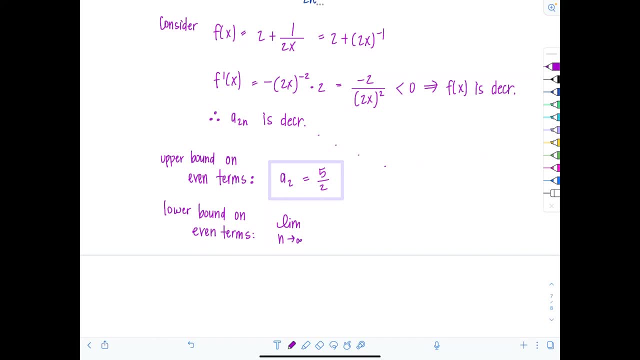 Time to look at a limit as n approaches infinity of just the even terms. So I'm going to look at the limit as n approaches infinity of a sub 2n. So that would be the limit as n approaches infinity of 2 plus 1 over 2n. 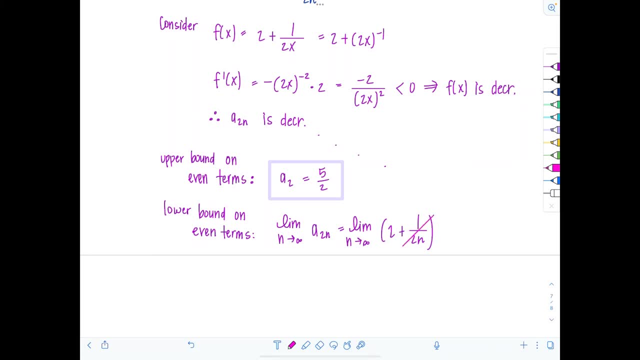 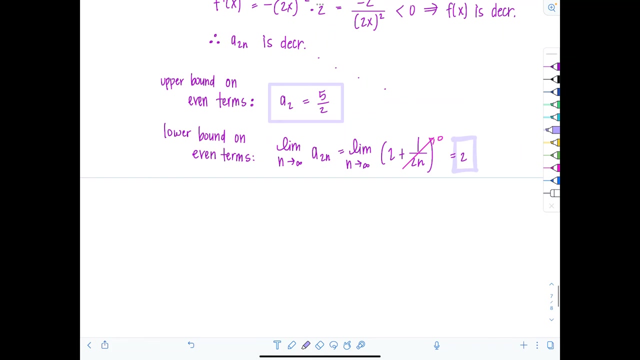 Well, hopefully it's pretty clear: 1 over 2n will approach 0.. So this limit is 2. And that means we do have a lower bound on those even terms. Okay, So the even terms: a 2n. 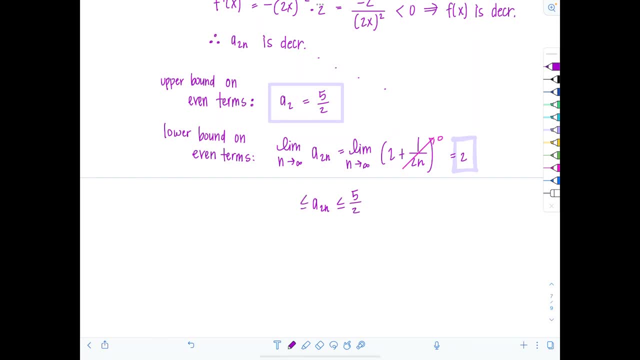 are always less than or equal to 5 halves, and greater than or equal to 2.. So the even terms are bounded. Okay, That's good, That's something. Now let's take a look at the odd terms. All right, How do I get an expression for the odd terms? 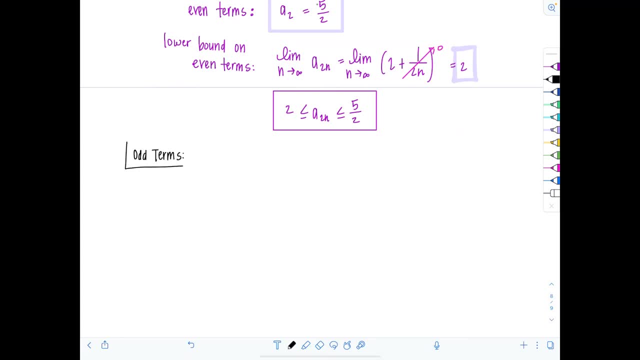 Well, a sub 2n represented the even terms And all you need to do is either add 1 or subtract 1 from an even number and you get an odd number. So it's up to you. You could use either a sub 2n plus 1. 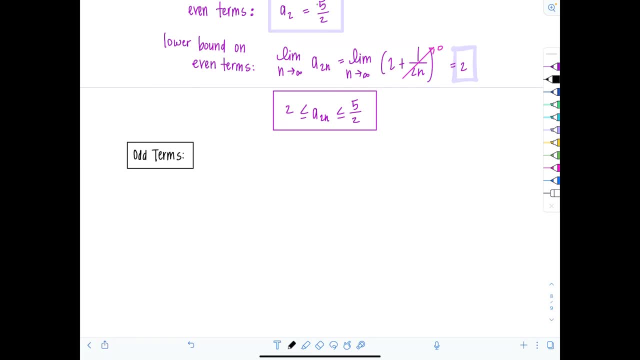 or a sub 2n minus 1.. I'm going to use a sub 2n or a sub 2n minus 1.. That way, the first term is going to be 1, a sub 1.. So this would be 2 plus negative 1. 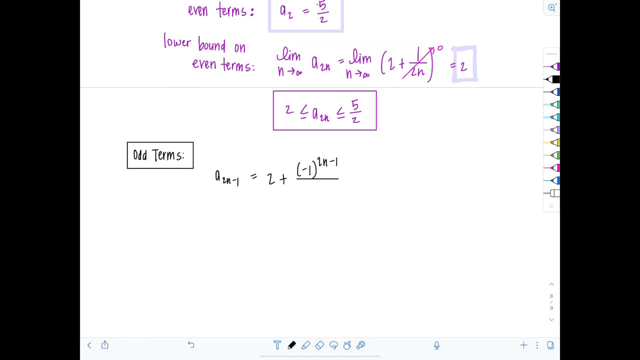 to the 2n minus 1 over 2n minus 1.. And then remember 2n minus 1, that's always going to be an odd integer. So negative 1 raised to an odd power is going to stay negative. 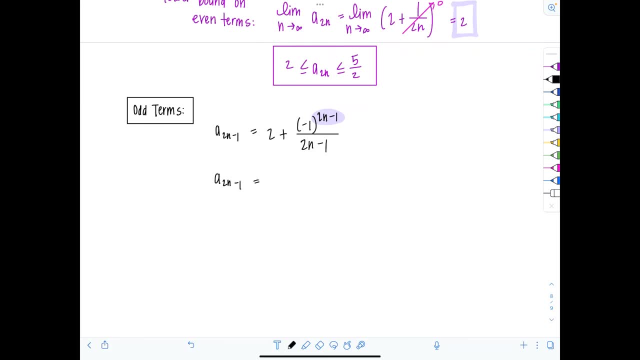 So a sub 2n minus 1 is going to be- let's clean it up- 2 minus 1 over 2n minus 1.. Make sense? Okay, I'm just going to box this because we're going to refer to it. 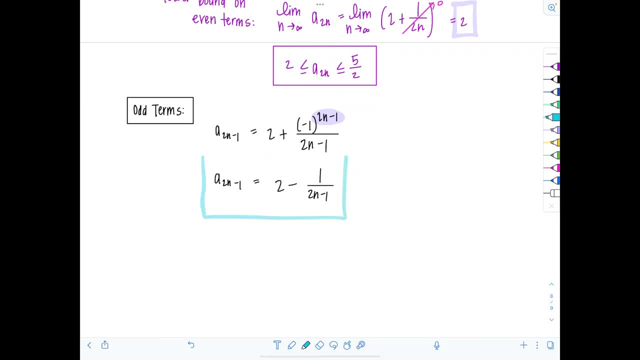 So again, I want to know if the odd terms are monotonic, Are they increasing or decreasing, And can I find bounds on them? So let's do something similar. We're going to define a function, So let f of x equal 2 minus 1 over 2x minus 1.. 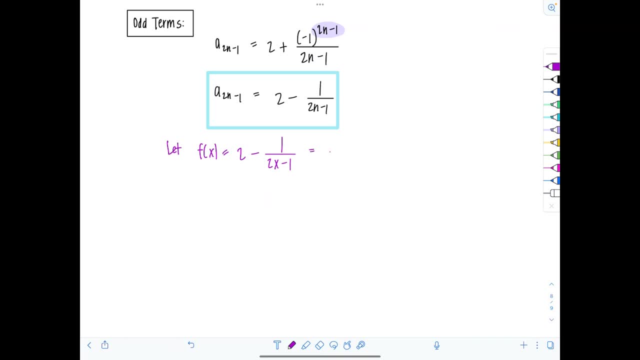 And I know I'm going to take a derivative. So let's rewrite that second term as 2x minus 1 to the negative first. Okay, So let's look at f. prime of x Derivative of 2 out front is just going to be 0.. 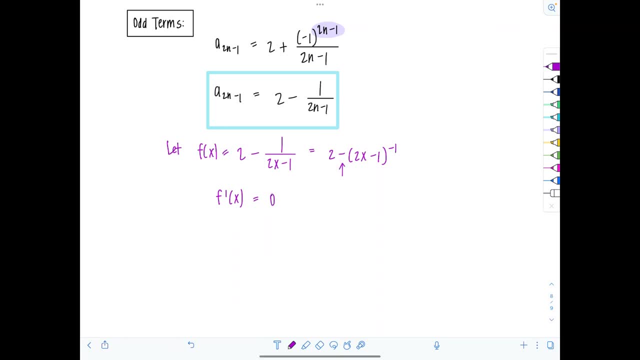 And then I'm going to have this negative, but then I'm bringing down that exponent in the front right. I'm going to multiply by negative 1.. So now it's going to become plus 2x, minus 1 to the negative 1.. 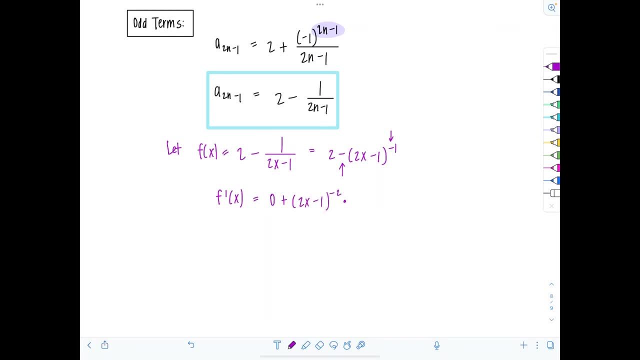 Plus 2x minus 1 to the negative second. And then, don't forget, we have the chain rule, So I have to multiply by the derivative of 2x minus 1, which is 2.. So now I'm left with 2 over 2x minus 1 squared. 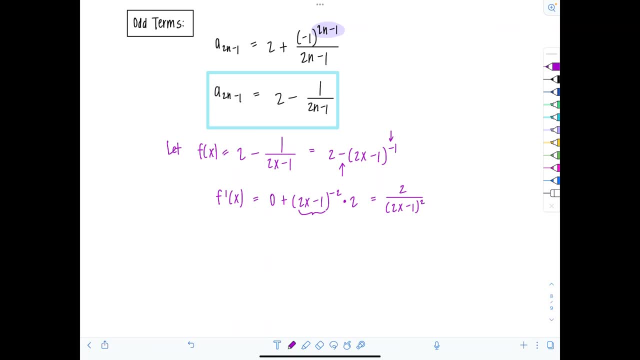 Hmm, Notice, in the numerator we have a positive constant Denominator. is some quantity squared, So this derivative is going to be 0.. If the derivative is always greater than 0, then that means the function f of x is increasing. 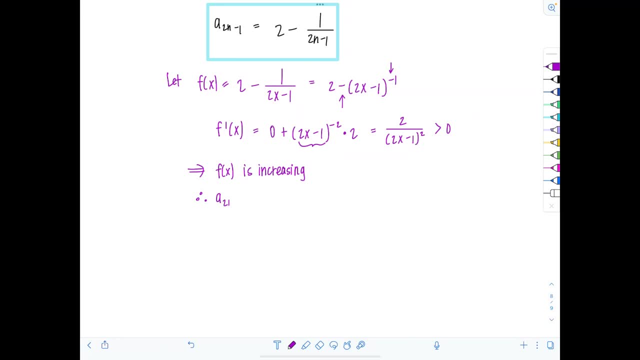 And therefore I can conclude that my sequence of odd terms, the subsequence, is also increasing. Okay, So let's think about that. So this subsequence of odd terms is increasing So that first term is a lower bound. That tells me a1 is a lower bound. 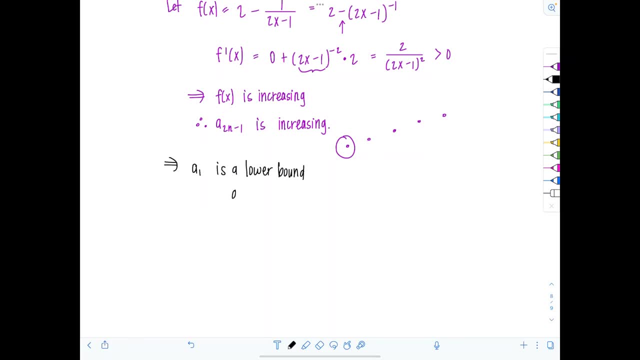 And what was a1?? We listed all the terms out earlier. a1 was positive 1.. Okay, Save that. Can I find an upper bound? So what I want to know is: do these terms just keep increasing forever and ever like that? 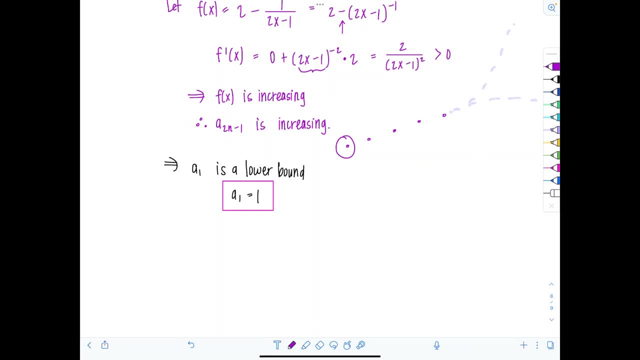 Or do they level off? How do I answer the question? I'm in calculus, I'm going to take a limit, So let's look at the limit as n approaches infinity of my subsequence of odd terms. So this is going to be the limit. 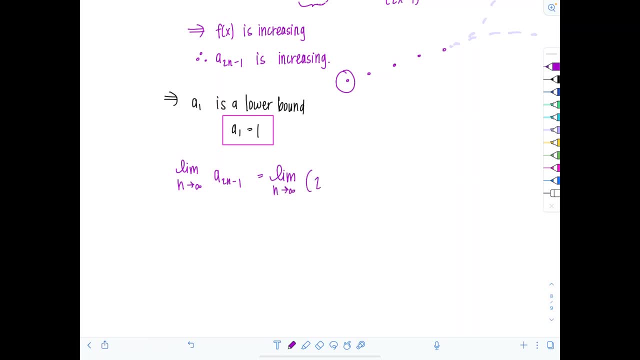 as n approaches infinity of 2 minus 1 over 2n minus 1.. Okay, Pretty similar to last time: 1 over 2n minus 1.. That's going to approach 0. So I'm just left with 2.. 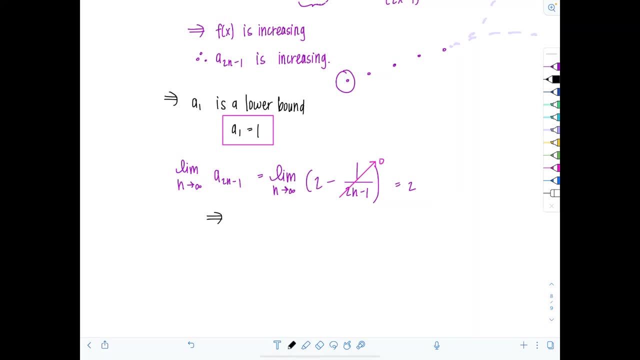 Ooh, this is good, This is good. So now that means 2 is an upper bound for the odd terms of my sequence, a sub 2n minus 1.. Okay, So we're going to summarize. now That means the odd terms are bounded. 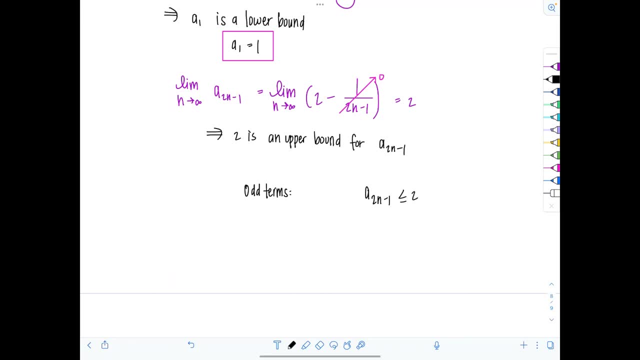 They're always less than or equal to 2, greater than or equal to 1.. The even terms, do you remember? They were bounded. also, They were bounded between 5 halves and 2.. So, putting it all together, what could I say about the sequence? in general, 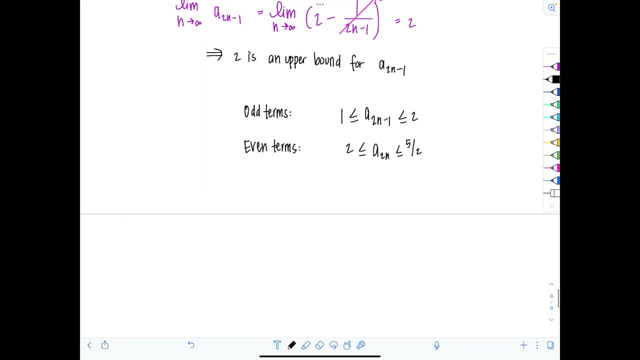 Is it bounded? Yeah, If we're not distinguishing between odd terms or even terms, I could say an is always less than or equal to. You're going to have to choose the larger of the two upper bounds for it to be still true.